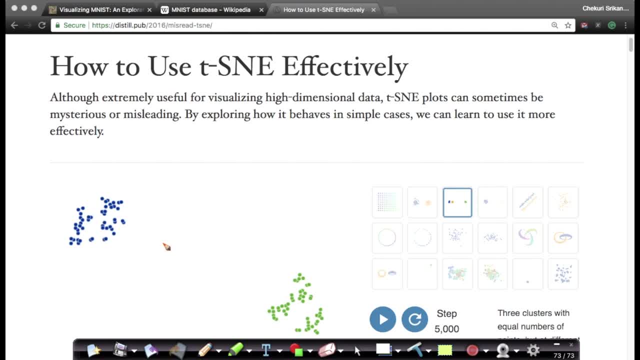 So, since we've learned about what t-SNE actually does, let's try to run t-SNE on simple data sets to understand how t-SNE behaves. So this is extremely important and for this purpose, I'm using a terrific blog called distilpub. Let me write it here: distilpub is a terrific blog. 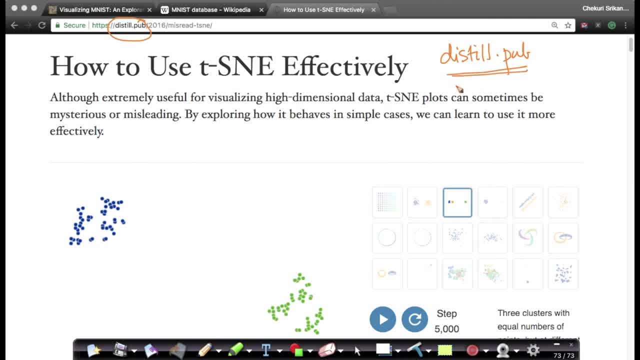 written as a collaboration between a lot of companies and spearheaded by a Google brain and Google research. So distilpub is a brilliant blog where they take state-of-the-art techniques in machine learning and deep learning and AI and they try to simplify it. They try to simplify it. 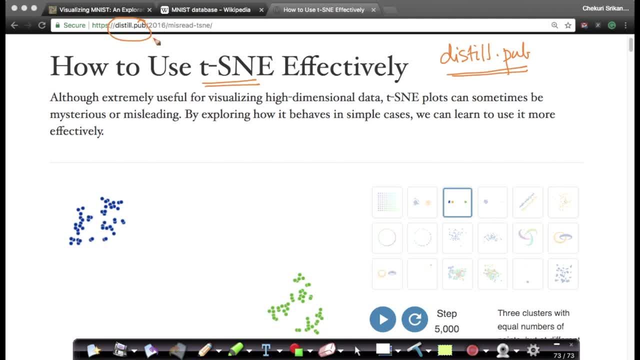 trying to give an intuition of how it works, and their first blog in, I think, late 2016, was how to use t-SNE effectively or how to interpret the results of t-SNE, and this blog was written and, by the way, distilpub is currently being collaborative. 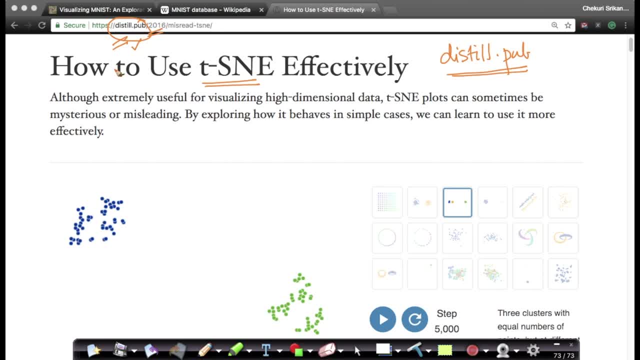 it's collaborative work between some of the best companies out there, like Google, OpenAI and a bunch of other state-of-the-art, state-of-the-art companies which are working on cutting-edge AI. This is a great work where they're trying to simplify, trying to give an 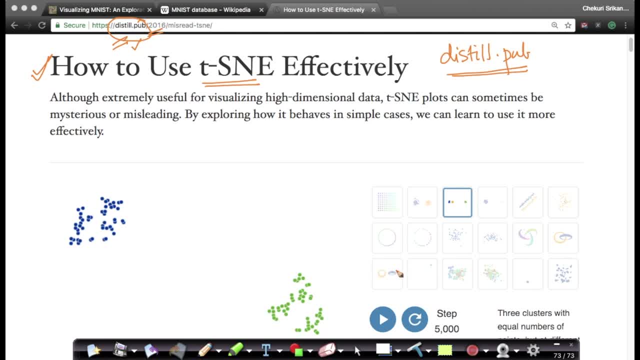 intuitive understanding, using examples, using live examples in some cases. So I think reproducing the results is very, very hard from my end as a single course developer. So I'm building on top of. I'm sitting on top of. I'm building on top of. I'm sitting on top of. I'm sitting on top of I'm. 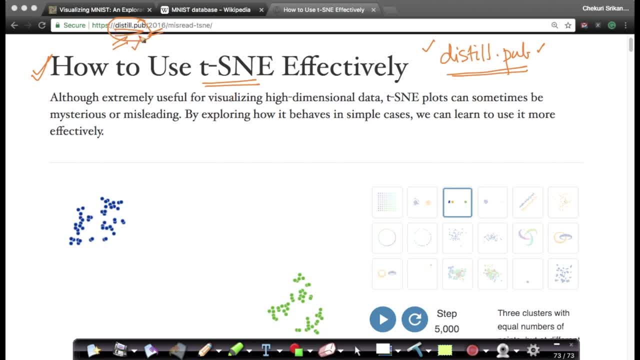 on the shoulders of standing on the shoulders of giants like people at Google Brain who have published this distilpub. I just wanted to credit the actual sources before I go and explain them. So let's see, let's see, let's see. So this page has a very, very interesting visualization. 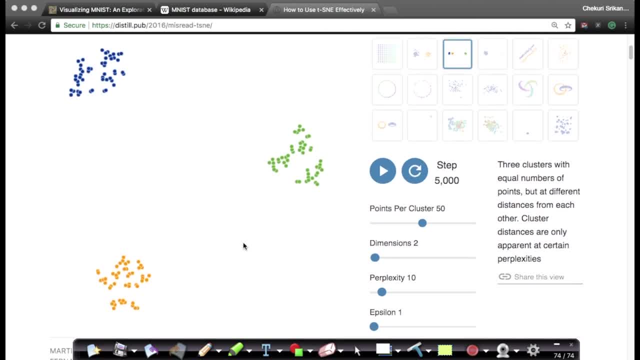 Okay, let's go and understand. So, before we even go and understand what t-SNE does, let's run it. So imagine I have a simple data set. Imagine that I have a simple data set. What we will do in this case is see what is dimensionality. 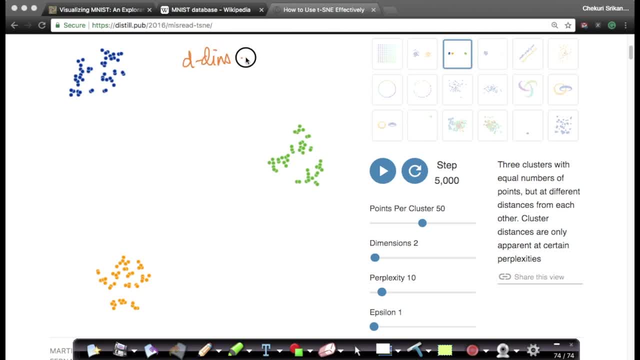 reduction, That I have a d-dimensional data and I want to project into d-dimensions Now to understand how an algorithm works, what if I make d equals to d-equals to 2.. Okay, so I have original data. This is only to understand. remember, this is only to understand. 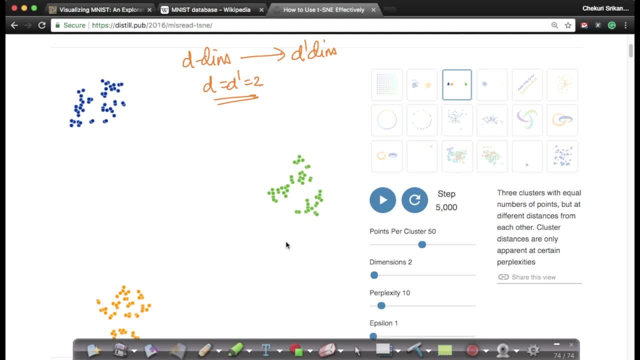 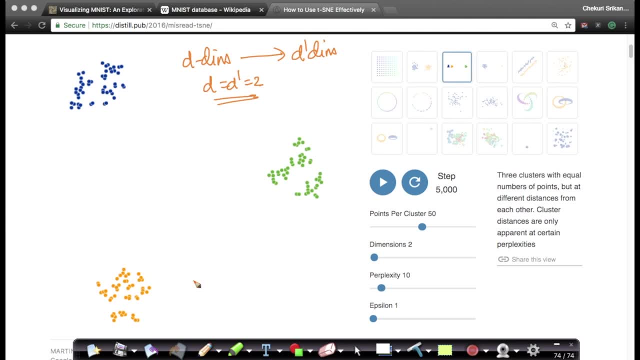 how the algorithms are working. This is only to understand. Okay, so what? what? what distilpub has done is it has taken a bunch of interesting data sets, So let's go through them. So this is a data set where I have three groups of points. 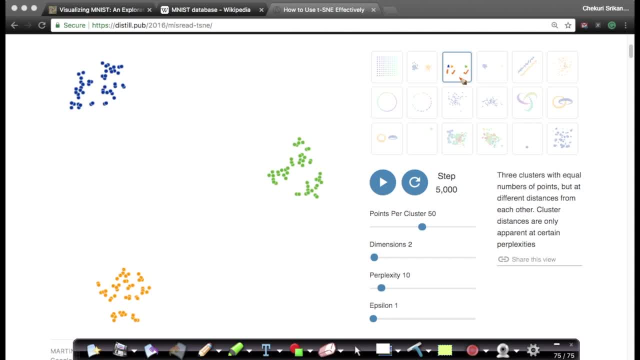 They're coloring them as blue, orange and green, Just so that I understand what's happening here. Okay, so so my data set is basically three groups of points in 2D space. Let's say this was feature one and this is feature two, And now I'm trying to embed them into a new space where this is f1 dash. 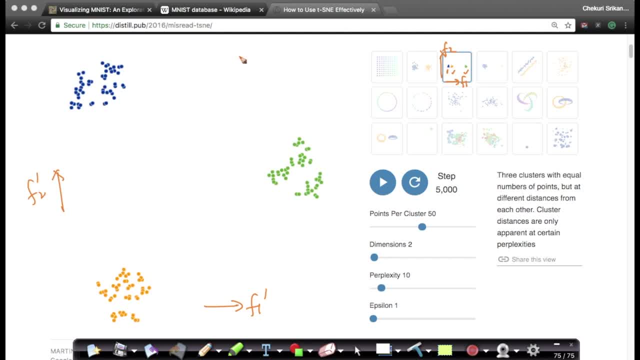 and this is f2 dash: 2 dash In dimensional reduction. I understand that you go from d dimensions to d dash dimensions, where typically d dash is less than d, but in this case we will make d dash equals to d, so that we understand how the algorithm is behaving internally. So if what we have here is exactly what we get, 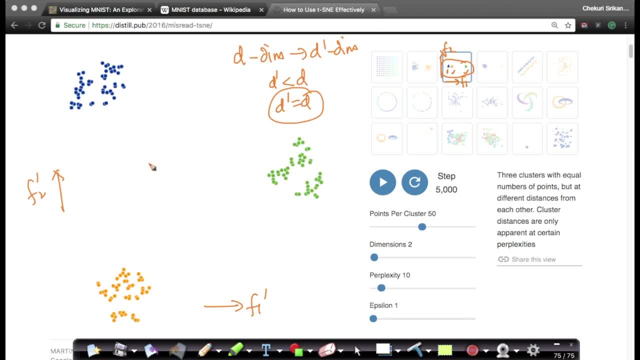 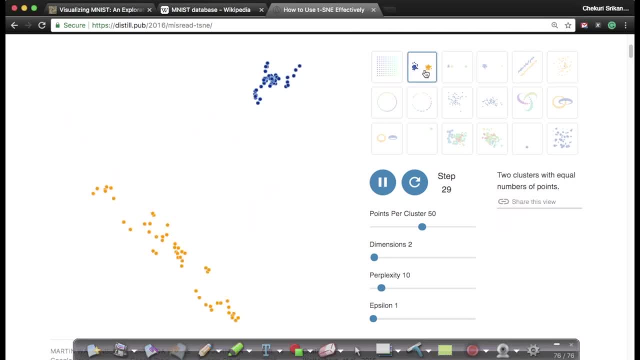 here as output, then the algorithm is working perfectly right. So here, in this case, distilled, dot pub has created brilliant data sets, for example. I can take this data set, for example: okay, So as soon as I click on this data set, this is the original data set and as t-sne algorithm. 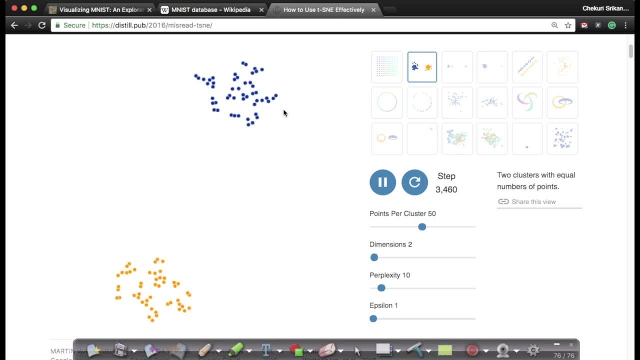 runs. this is the output that I get eventually, right? So they're actually running the t-sne algorithm in the browser right here using javascript. okay, So imagine if my original data set was like this: two parallel lines of points. okay, So t-sne basically runs. so t-sne. 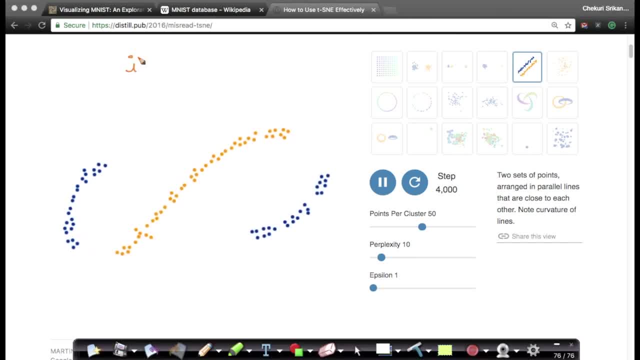 is an iterative algorithm. t-sne is an iterative algorithm, which means t-sne tries to process all the data in iterations and eventually it wants to reach a stage. eventually it wants. so it goes. it does the first iteration, second iteration, third iteration, so on, so forth. okay, and eventually it wants to. 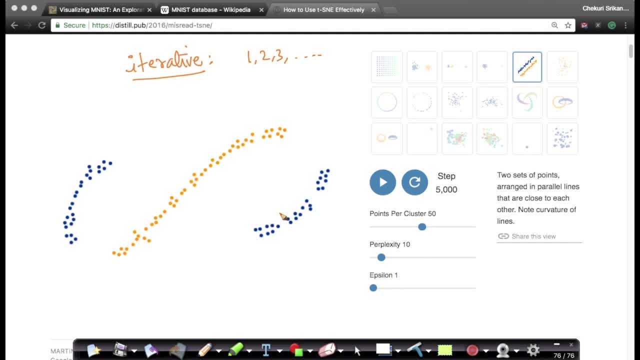 reach a stage where the clusters are no more moving. At every stage it tries to move the points. at every stage it tries to find an embedding. okay, and with every stage it will try and improve the embedding so that it's as good as possible, so that it's trying. 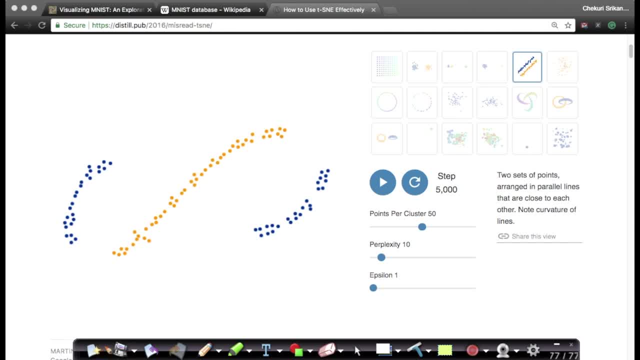 to preserve as many neighborhoods as possible. okay, So now let's take this example. so there are. so each of these data points, for example, if you take these two parallel lines, okay, there are 50 points per cluster, so there are 50 points here. there are 50 orange points. 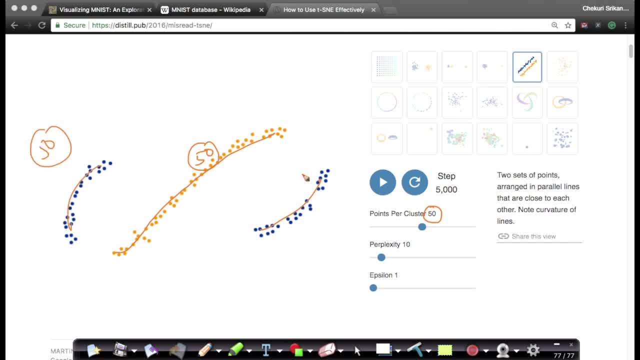 and there are 50 blue points. okay, between these two blue points, there are 50 blue points and there are 50 orange points here. okay, There are two most important parameters. there are two most important parameters of your t-sne. the first parameter is called perplexity. the second parameter is called step size. let 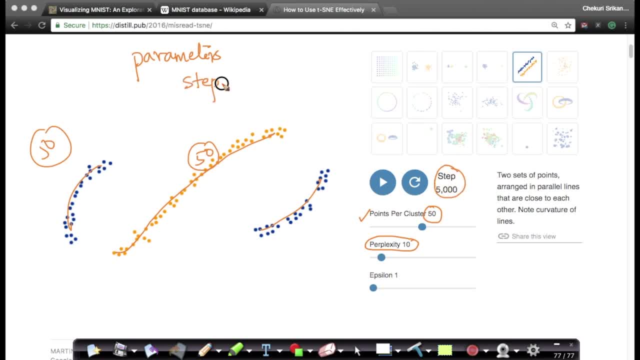 me explain you what they are. so step size: step size is basically the number of iterations. so just remember that with every iteration you're, you're going to find a better solution right For the iterations, because what, as I told you, t-sne is an iterative algorithm where 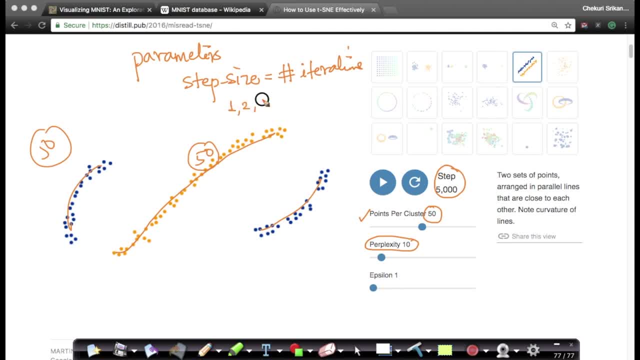 first, it will iterate through all the points in iteration 1, iteration 2, iteration 3 and in this case we go up to iteration 5000. right, and in every iteration it tries to find a better solution. for example, if I just run this right now, let me just run this, okay, let. 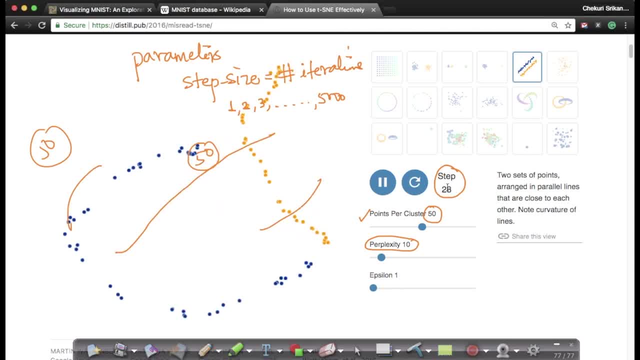 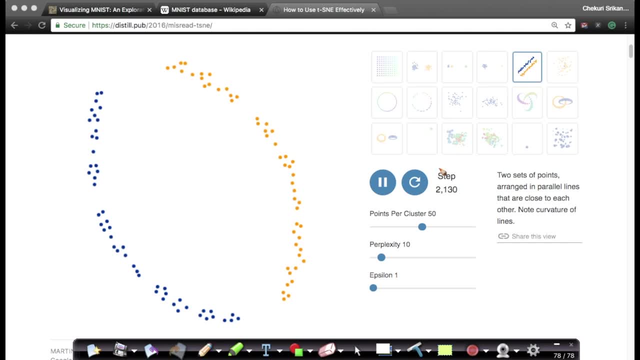 me just run this. so if I just rerun it, okay, see, as the step size increases or the iteration increases, my result is getting better and better. Let me just erase this right now. So notice this as my step size, as my step size. so let me refresh it again, my original. 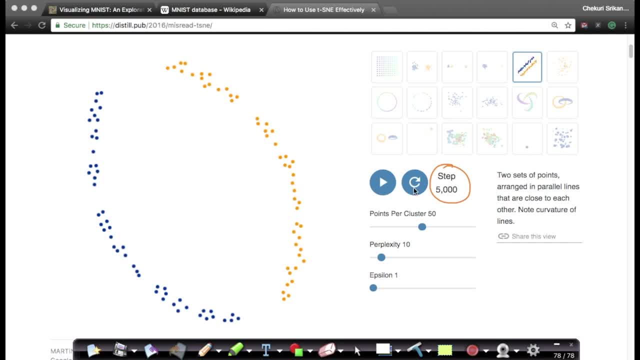 data is two parallel lines of blue, blue points and orange points. now let me just see: okay, so, okay. so at iteration 14 you don't get the shape right if I continue. by the time I go to iteration 100. right, I'm getting some parallel line type structure right if I keep going. 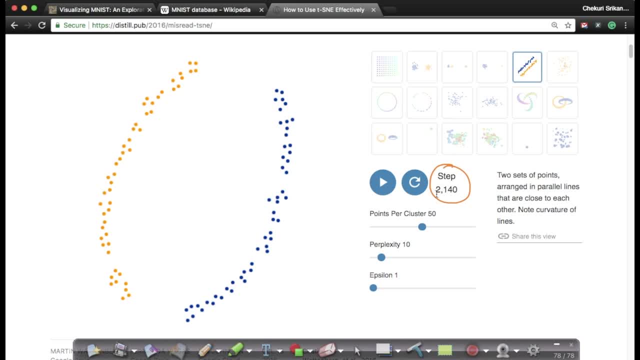 on, if I keep going on, okay At iteration 2100, right, Okay At iteration 2100, I get the shape, okay, which is sort of like two parallel lines, right, which is sort of like two parallel lines here. okay, with some arcing here, which is which is interesting. 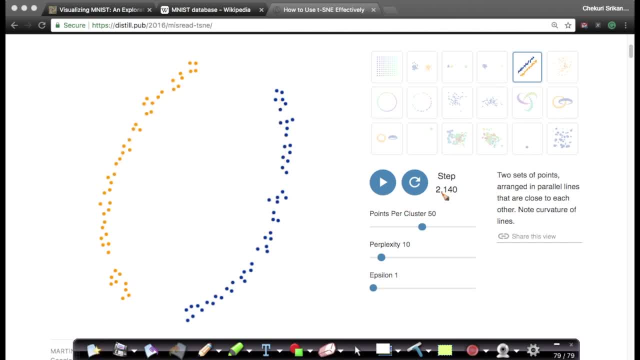 we'll see why that happens. okay, but eventually, if I continue, if I continue from 2000 iterations, if I keep going ahead, okay, okay, so as just look at this as the as the step size or the iteration number increases, the shape is stabilizing and now the shape doesn't change much. we have 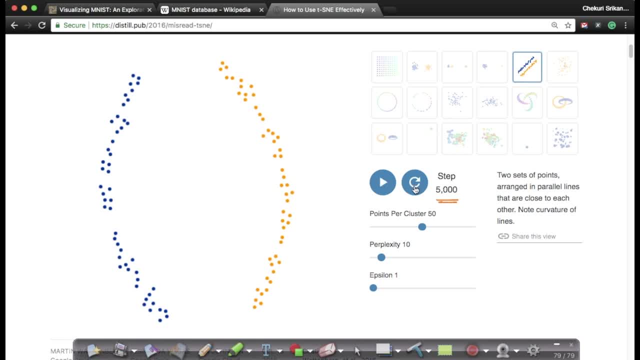 reached about 3000 iteration and the shape doesn't change. Okay, Let's see that once again. just to understand this. just notice: as the step size increases, this shape starts getting more and more stabler. it will start moving less and less. okay, let's. 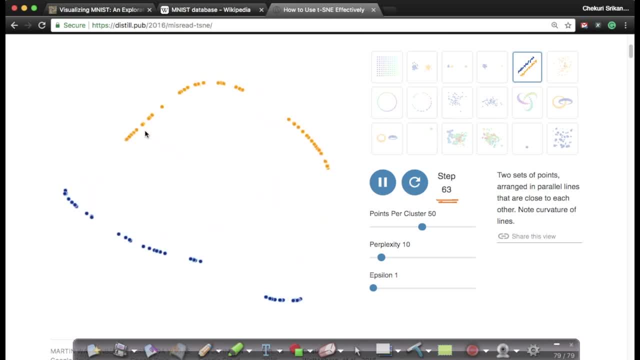 let's see that. okay, as it increases. yes, yes, it's trying to. now it's trying to move towards the best shape, which is actually two parallel lines. okay, we have reached about 2000 iterations. it's it's almost stopped moving now. okay, now it has converged at the end of 5000 iterations. 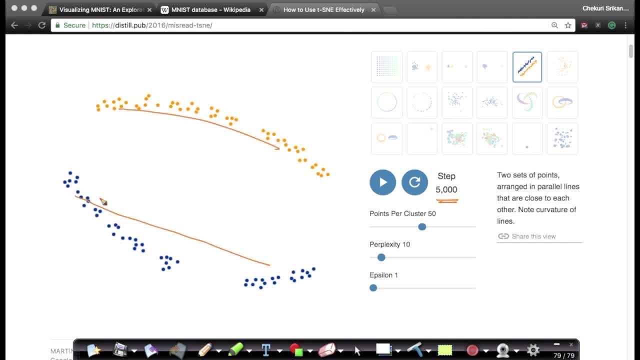 you almost get a structure like like, like this, with some with some parallel lines, okay, Okay, Okay, Okay, Okay. So now you have to get some arcing. this is very similar to the actual underlying structure of data, right? so similarly, if you, if you look at so that that's what step size means. so 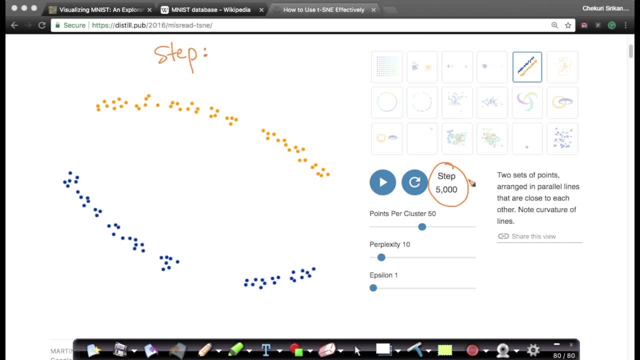 step size or step. here it's called step, not step size. sorry, here step is nothing but number of iterations you are performing, and remember that more the number of iterations, the better is the solution. okay, and you should keep iterating till till the time the shape doesn't change. 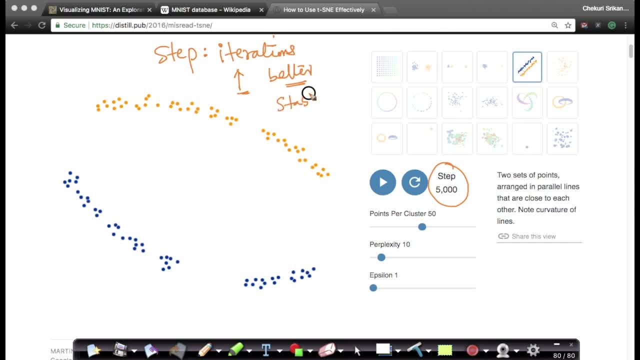 much that's called till the time it reaches a stable consciousness, Okay, configuration. what is stable? it means this shape, this shape is no more moving. we saw right a while ago that after 2000 iterations this shape hasn't been changing much. okay, that's so, that's one. 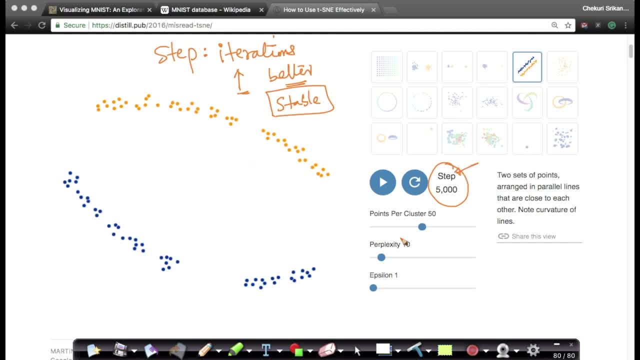 parameter. it's called the number of iterations or step in this block. the second or the most important parameter of t-SNE is called perplexity. let's understand what perplexity means. you can think of perplexity roughly or loosely. roughly or loosely as the number of neighbors, the number of 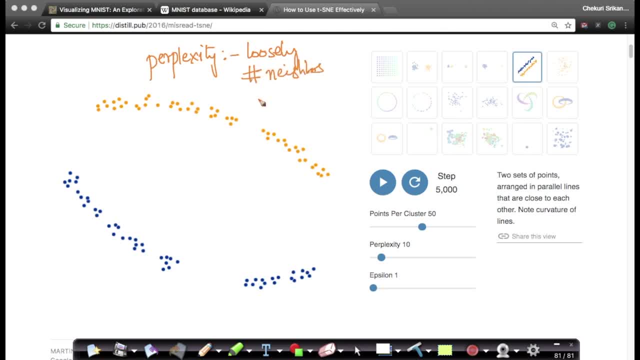 neighbors: number of points or number of, instead of using neighborhood as a distance measure. so if I have this, instead of saying that this is my neighborhood, what if I say I want to preserve distance of five of my nearest neighbors? okay, five points. so if I say, if I, if I make my perplexity, 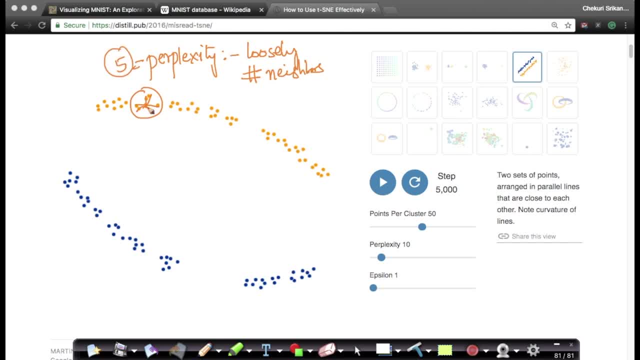 equals to five. what it tries to do is, for every point, it will take five points. it will take five points which are closest to it- okay, which are these five points? and will try to preserve these distances, instead of preserving a dist in a distance of d. instead of doing that, it says: 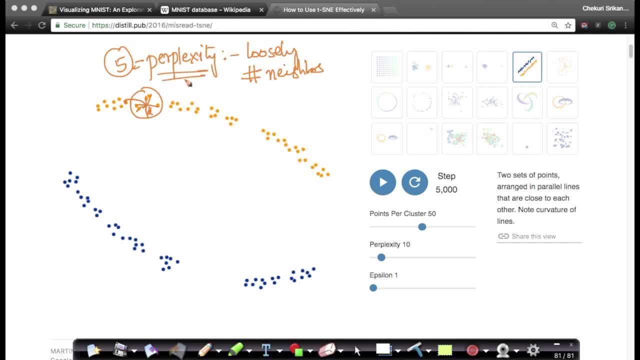 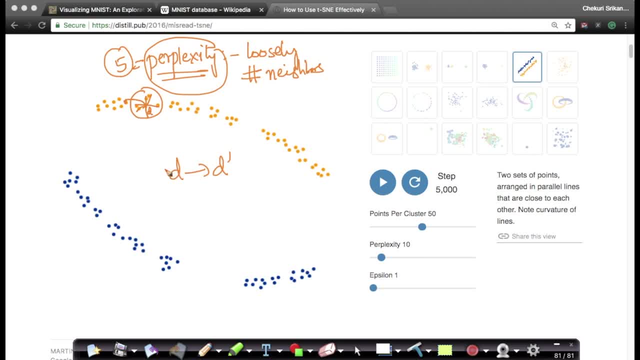 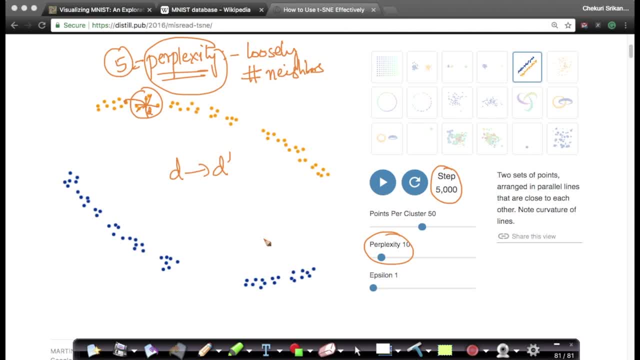 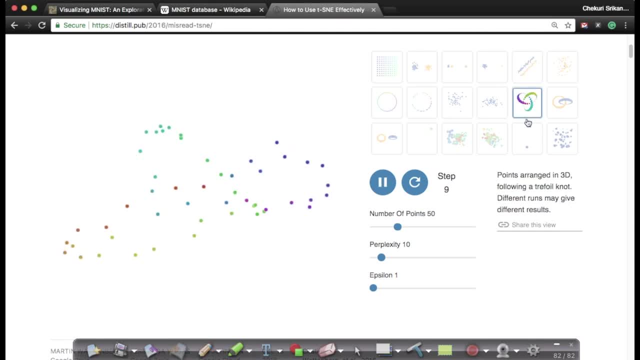 a little more time than usual for us to cover this. this is brilliant. block. okay, let's go. let's go through examples now. we'll come back to revisit these examples. this is brilliant. suppose if I set like this right as I keep, eventually I'll get a data set. okay, you can see the structure here. 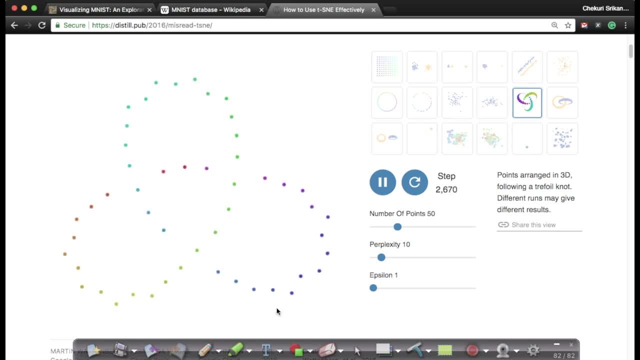 right. you can see this, this knot like structure evolving out of it. so all of your violet points are here, just like this. all of your light green points are here, right. all of your darker green points are here, or reddish green points are here, right. so by 5000 iteration I get the structure of 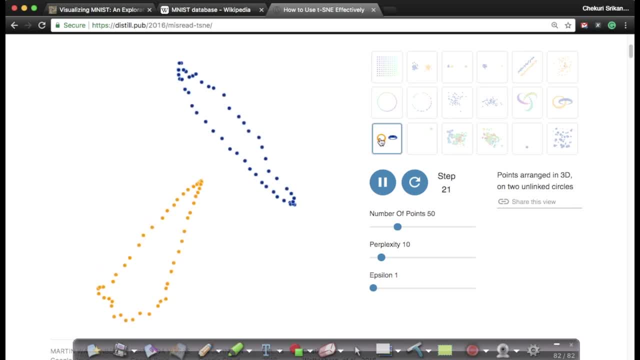 the data right. similarly, if I have my data set like this- two rings right- eventually I've reached a two-dimensional which is two rings, and I've reached it even just by 1000 iterations. okay, so the two most important parameters, just to reiterate, are step size or sorry step, or number of iterations- sorry step. 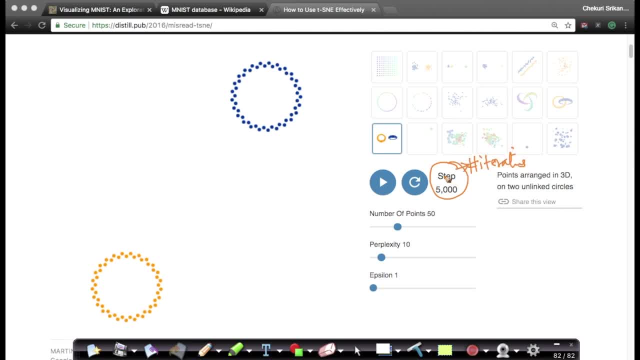 size has a different meaning in optimization. sorry, it is step, so we I typically call this iteration. that's why I'm getting confused between step and step size. sorry, so let's just call it number of iterations and perplexity. okay, two most important. perplexity says how many data points in 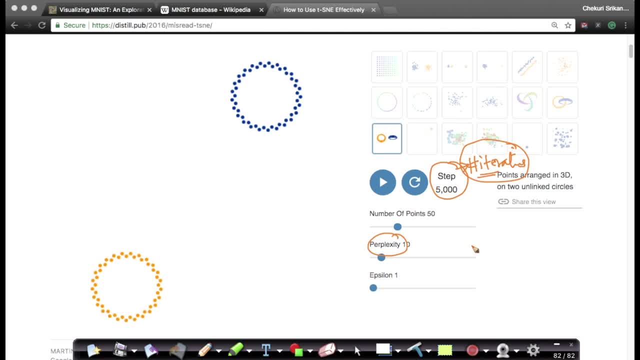 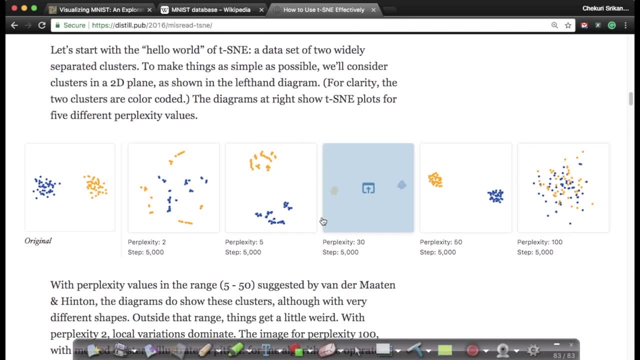 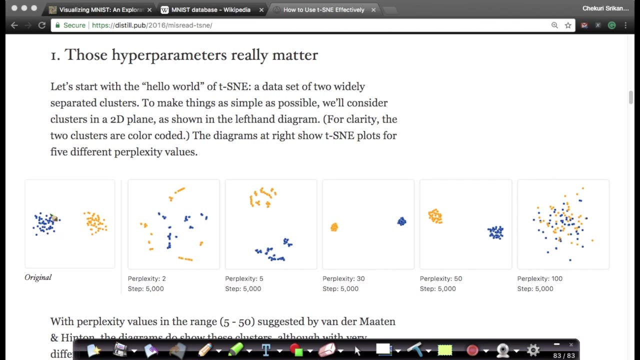 a row whose distances I will try to preserve when I do a dimension introduction. okay, let's go through examples now. this is this is the most interesting part. so our first example is this: okay, our first example is: let me change the color here just in the. okay, I'm taking dark green here, suppose, if 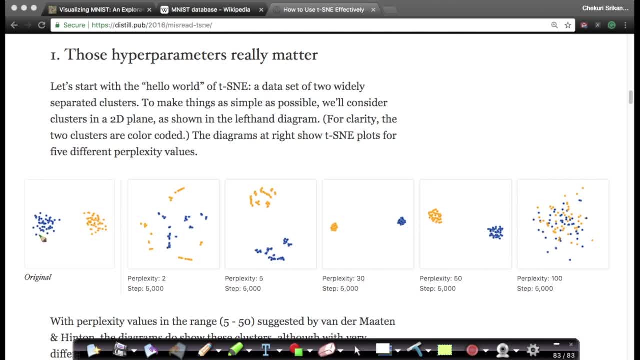 I have because orange points are already there. I don't want to mess it up. so imagine: originally I have my data set like this: I have a bunch of a bunch of blue point and a bunch of orange points. my step is 5000, which means I'm running it for 5000 iterations. right, this is very, very important. 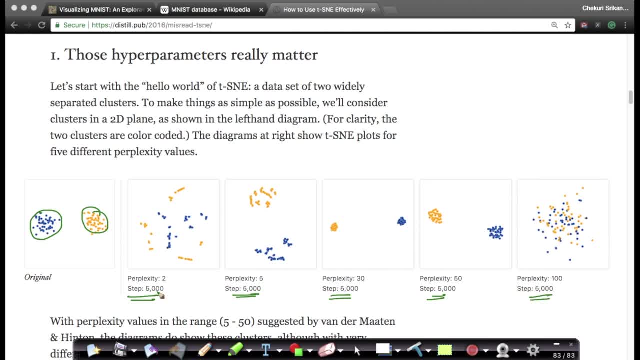 okay now, the first thing that you'll notice is if I make my perplexity very low, if I keep my perplexity to, which means I am trying to preserve only distances, of distances to two nearest neighbors or two points which are which are the closest to a given point. okay, if I make my 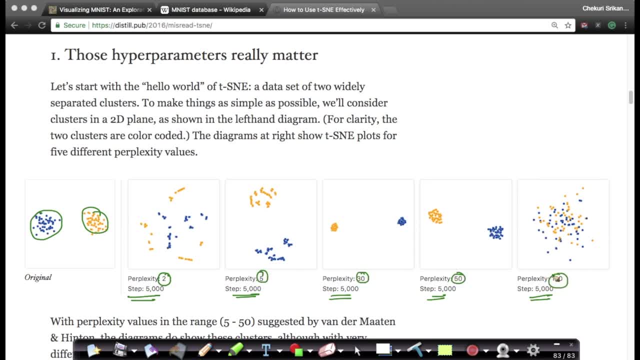 perplexity 5, 30, 50 and 100, and remember I have 50 blue points here and 50 orange points here. okay, that's how I constructed this data. when perplexity is very small, say, and we want to, we want to read, we want to get this structure right, which you can see, and perplexity equals to 30 and 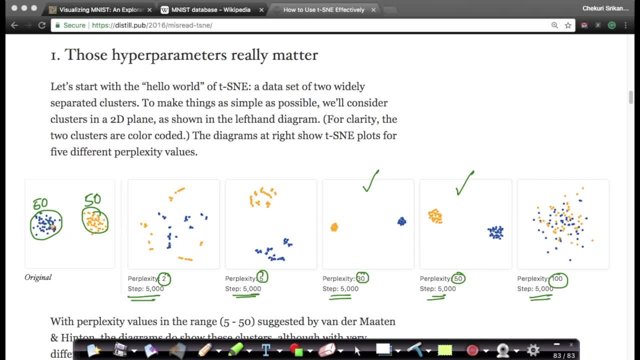 perplexity equals to 30 and 50, you're getting roughly this shape. roughly, not necessarily exactly, but roughly this shape. right now comes interesting part: when perplexity is very small, you are getting a structure like this structure. if these are your blue points and if these are your green orange points, this structure is completely absurd. so when perplexity 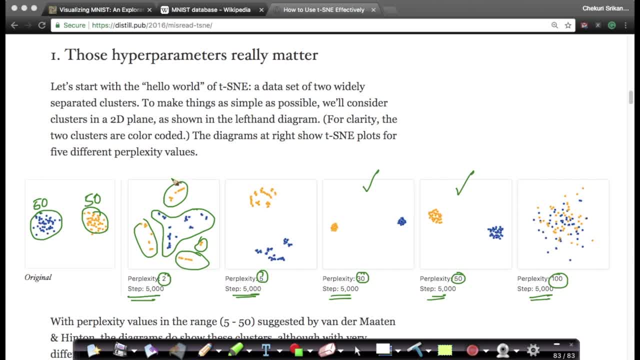 is small, the results you get can be crazy. right, as perplexity increases. as perplexity increases, right, your shape will start to get much, much so sensible again. this is not sensible. this seems more sensible, right that you have two groups of points. so, for example, if this is some high, 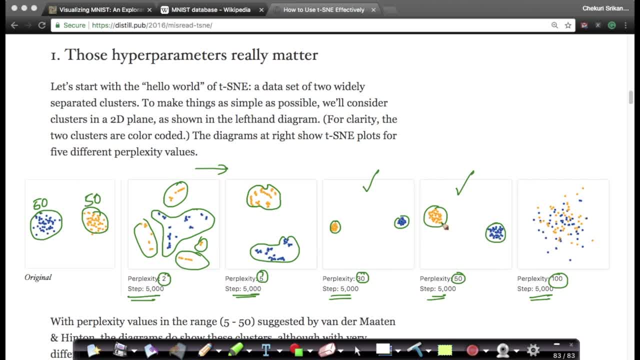 dimensional data. as soon as you visualize this, I say, yes, there are a bunch of points here, there are a bunch of points here and they're well separated. okay, now there is a catch here. so the lesson from this, the lesson from this is number one: always run your t-snee with multiple 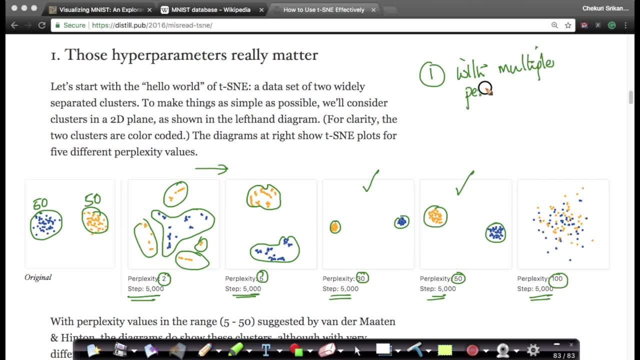 with multiple perplexity values. perplexity values: okay, keep increasing the perplexity value. never say perplexity equals to five. seems okay. no, don't do that. please don't do that. run various values of perplexity and she see the shapes that are more stable. so as soon as you. 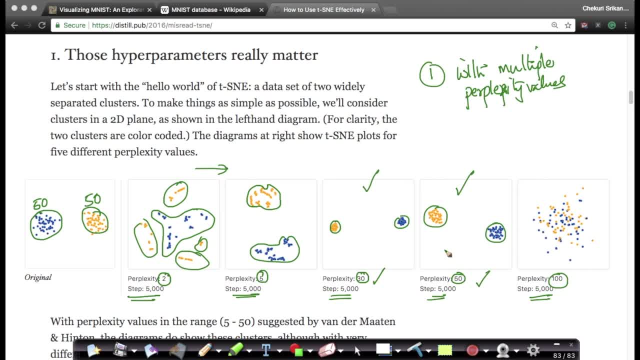 see this okay between 50 and 30. this table is fine. now comes an interesting aspect. so first lesson is: never fix one perplexity value. always run your t-sne for multiple perplexity values to understand the actual shape. so never run your t-sne only once. that's the most important thing. 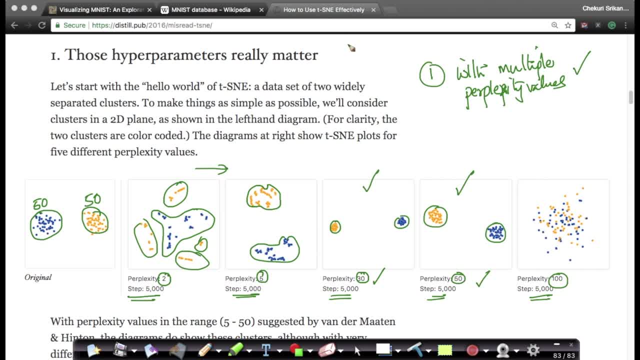 so when, when you run t-sne you're given, you give two parameters, you give perplexity and number of iterations. okay, never run your whole t-sne. your t-sne function right in scikit-learn- that we will see- has these two. it has many other features, of course, but these two are the most important- never. 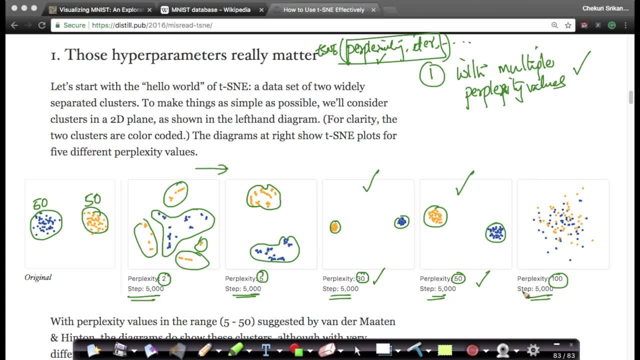 run it with one perplexity value. always try to run it with multiple perplexities. now here comes one more interesting thing. when i make my perplexity equals to 100, my total number of points are 100. right, when i make my perplexity equals to 100, i get a mess. this is literally a mess that i that i. 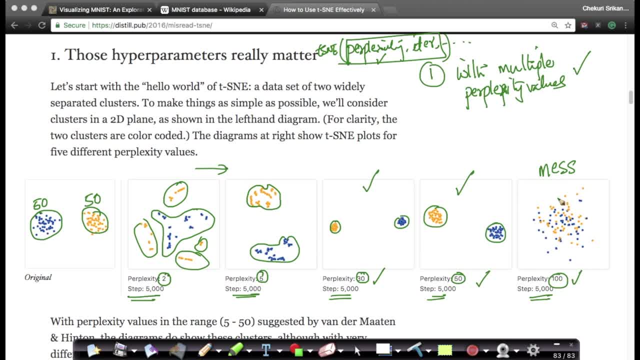 end up in now. why is that happening? see when, when, when i'm trying to preserve distances for every pair of points. see when perplexity equals to 100, which means for it- and i have only 100 points here, right, what is? my total number of points is only 100, 50 plus 50. so when you make your perplexity, 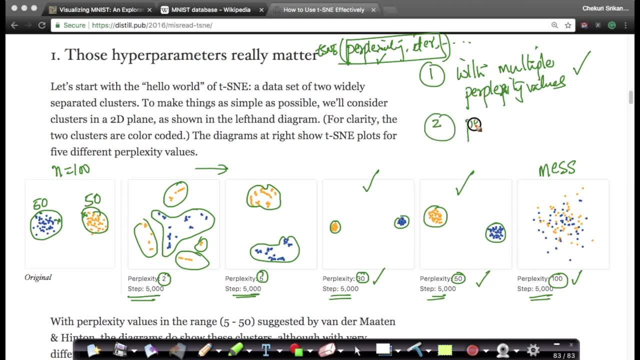 the second most important lesson is: if your perplexity equals to number of data points, okay, you'll simply get a mess. so always try to keep your perplexity less than your number of data points. so the lesson learned from this is: whenever you run your t-sne algorithm on a data set, 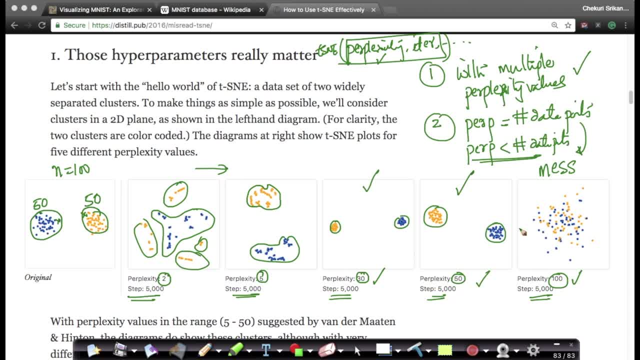 try multiple perplexity values till the time, but never put perplexity equals to n or the number of points. so you can think of this in another way: perplexity, so t-sne. as we learned, does neighborhood embedding right, but if i make my, perplexity equals to number of data points. 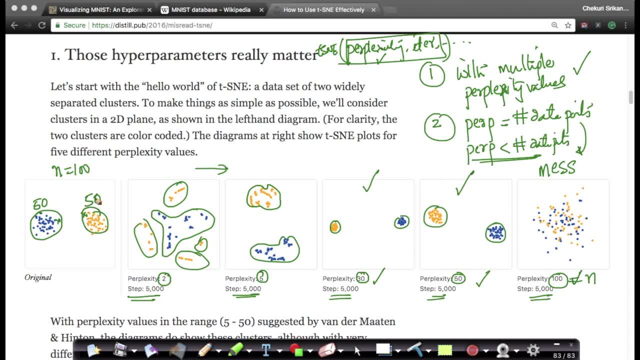 it's no more preserving just the neighborhood. it's trying to preserve the whole data set, the whole structure of the data set, and where it does a, it does a terrible job. okay, so this is. this is one of the first lessons that we need to learn from from tc. okay, so please. 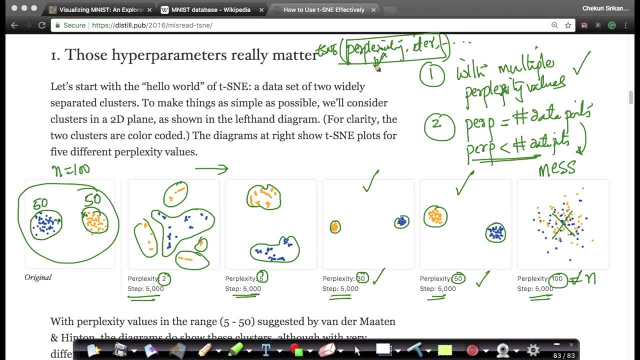 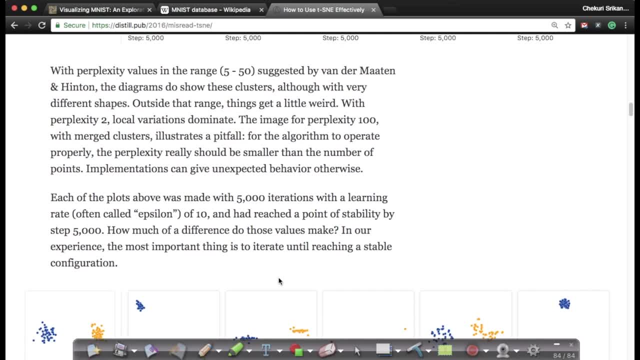 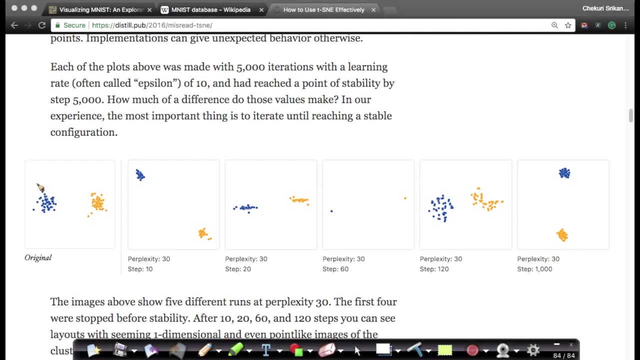 whenever you run t-sne on a data set, please run it with various values of perplexity. and that's the first lesson. the next important thing is: sorry. the next important thing is: okay, what if i keep my perplexity constant? so if you look here, so again, same data set i kept. 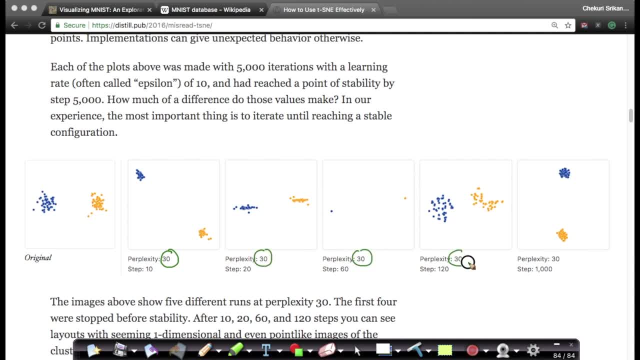 my perplexity as 30 every time. okay, but i'm changing my step here, which means i'm changing my number of iterations. so my number of iterations or step, okay, i'm increasing, stepping with only 10 iterations, 20 iterations, 60 iterations, 120 iterations and 1000 iterations. okay, you'll. 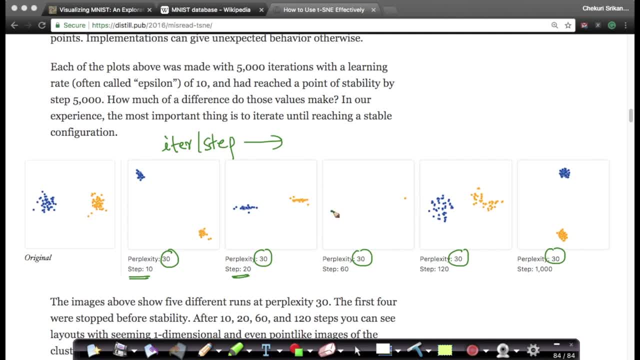 notice that this, this seems absurd. right that i have all the points grouped in a small area here. so the lesson is always: run your iterations till the time the shape doesn't change much. okay, so when i start here by by 10 iterations, i got some structure like this: but don't stop here, let it run till the time. so probably a thousandth. 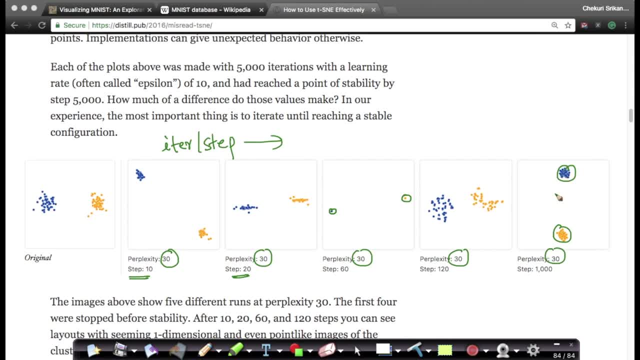 iteration you get a shape like this and in thousand one titration these points don't more, don't move much, so always run your t-sne. so when you are analyzing t-sne, it plot your t-sne for various values of step or iteration, okay, and see if this, if the shape, 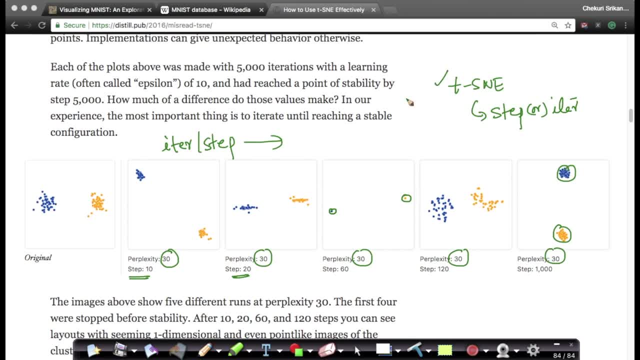 has stabilized. okay, so that's very, very important. so first lesson learned was always always run t-sne for multiple values of perplexity. find the right type of perplexity by keeping your number of iterations large and then change the iteration now to understand whether the shape is stabilizing or not. this is a very important lesson. okay, there is one more. 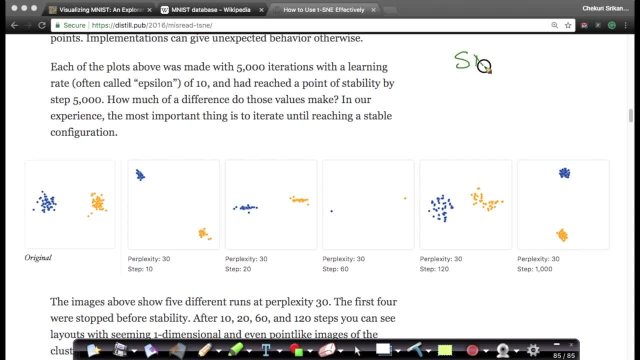 small catch with t-sne. so t-sne, i explain you what is neighborhood embedding? right, okay, neighborhood embedding. we understood t distribution to solve the crowding problem. why stochastic? stochastic basically means probabilistic, if i mean that's one way of thinking about it. probabilistic. so if you run t-sne, if you run t-sne multiple times, you might 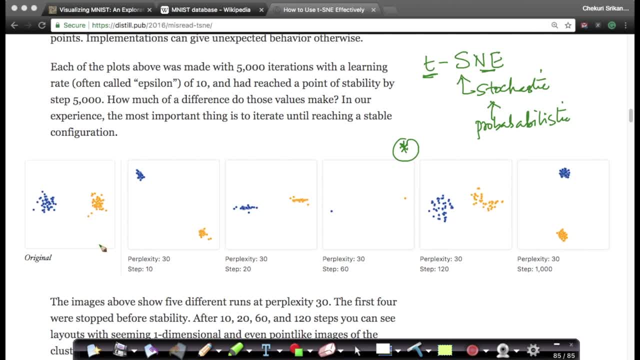 get small. so if you run t-sne on the same data set with the same perplexity value, let's say, same step or same number of iterations, you could get. you could get slightly different results, slightly different results. that's because t-sne is not a deterministic algorithm. what's a? 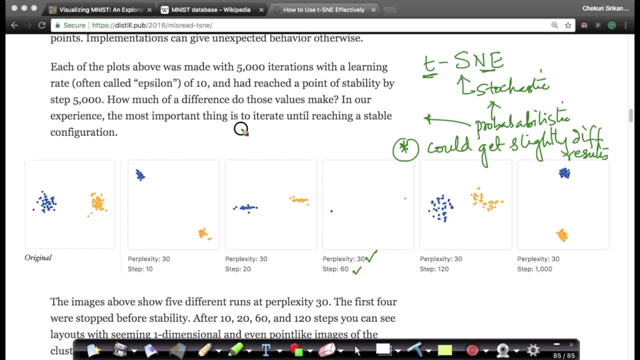 deterministic algorithm when the output: if, if i have an algorithm, if i give it some data every time i run this algorithm. if i get the same value, that's called a deterministic algorithm, every time i run. if i get a slightly different value, that's called a probabilistic algorithm. 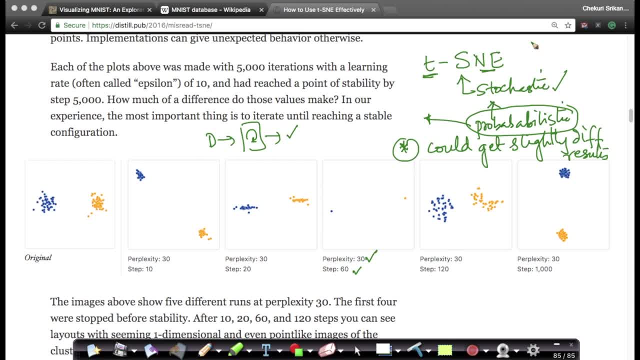 or a stochastic algorithm. okay, so t-sne is actually internally- the internals of t-sne- is actually a probabilistic algorithm. so that's why t-sne doesn't do just neighborhood embedding, it does a probabilistic or a stochastic neighborhood embedding. so that's the other. 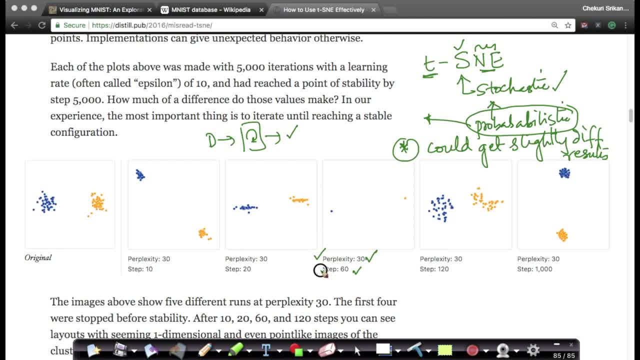 lesson. so if you have learned what is the right perplexity and the right number of, so let's assume here you learned that perplexity 30 is good and number of iterations 1000 is good. the next lesson is: if you run it multiple times you may get slightly different results. 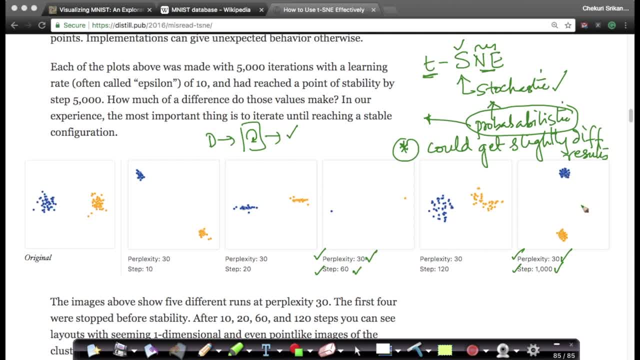 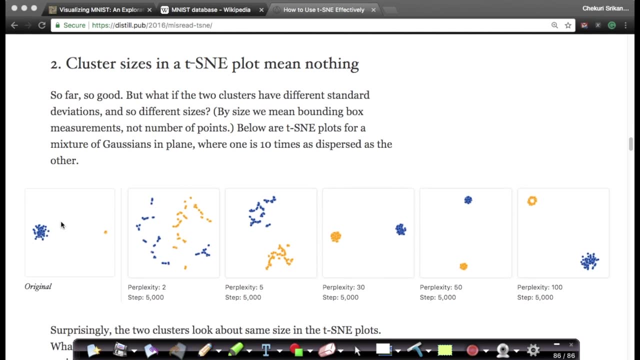 it's always good to see the results being run multiple times, because every time you run there is a small difference in in what the output is okay. so so that's the next important lesson now comes. now comes a scenario like this: now imagine that i have 50, 50 points. 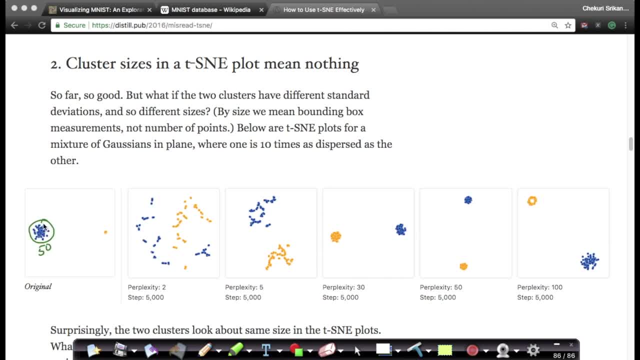 i have 50 points here- blue points that are- and i have 50 orange points here. these orange points are very, very dense because i've packed all my points in a very, very small area, right right. so this cluster size is small, or this group size, because the variance is small here. okay, 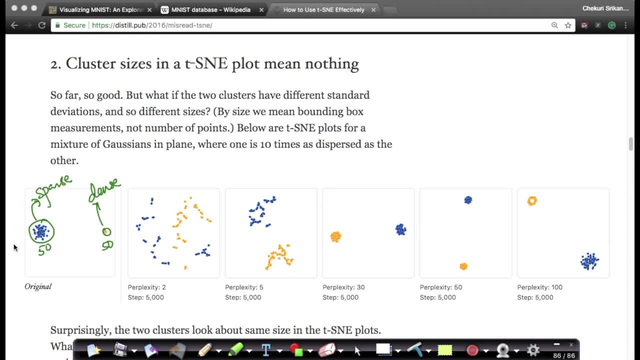 these are sparse. these are sparse points, right, so now, now let's, let's see what happens as i change my perplexity and my so i'm keeping my step size very large, 5000 here, which is good. okay, let's assume i've determined that after 5000, by the time i reach 5000 steps, the shapes do not change. 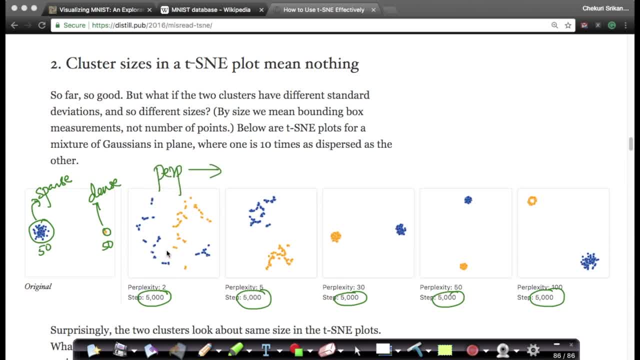 much now i'm increasing my perplexity here. i'm doing everything from two, five, thirty, fifty, etcetera, etcetera. now the one thing you realize quickly is, as i'm going: okay, my 30 and 50 look good. but there is one big catch here. if you see the shapes of my clusters, the orange points and 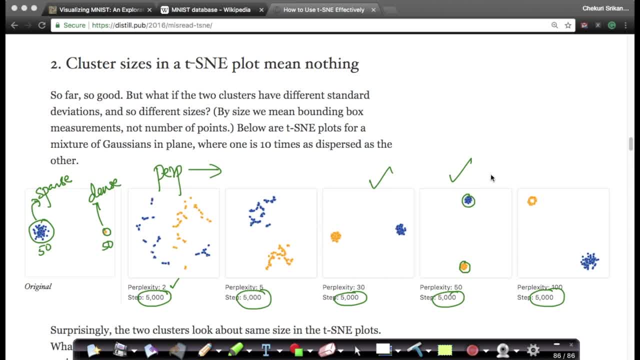 my blue points. both of them typically have the same density. This has the same density almost as this, But my original data set. my orange points are much more dense and my blue points are much more sparse. So one of the things that t-SNE does internally. 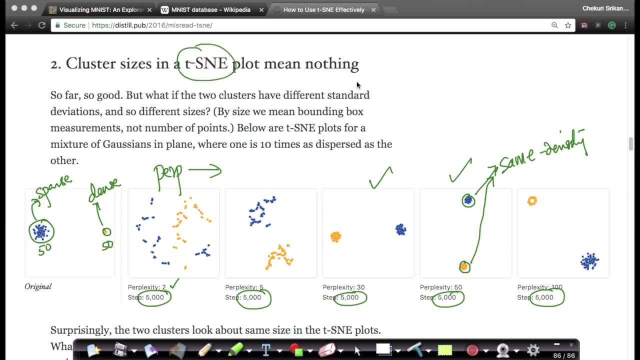 one of the things that t-SNE does internally is it basically expands. it basically expands dense clusters or dense group of points, and it contracts or shrinks. it shrinks or contracts sparse clusters. So what t-SNE is trying to do is t-SNE. 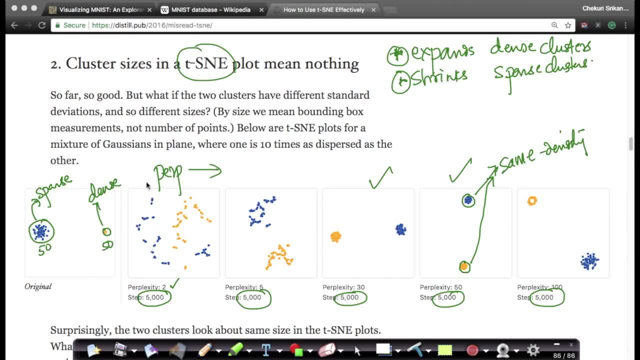 because of the way the mathematics inside t-SNE work. what t-SNE tries to do is it tries to because it's also a stochastic neighborhood embedding algorithm. one of the things that t-SNE does is it shrinks. so these are sparse points, right. 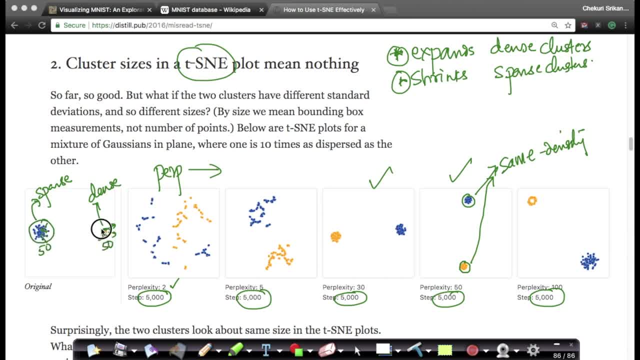 It shrinks these points and it expands these points because they're very, very dense, such that the densities of the densities of both of my groups of points are roughly similar. So one of the things that you cannot read from t-SNE is whether a cluster is dense or sparse. 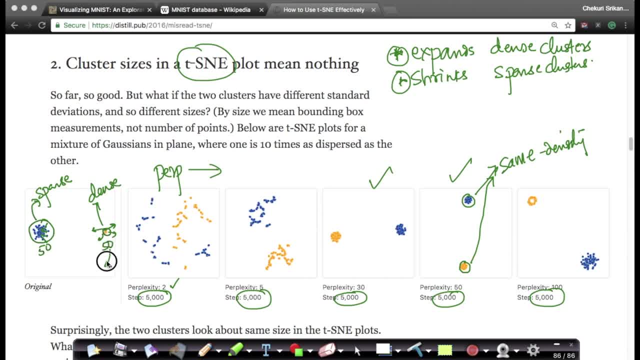 You cannot get cluster sizes, okay. This is called a small cluster because it's very, very tightly grouped. This is called a large cluster, right, So t-SNE. so imagine this was the data. Imagine if we've never shown this. 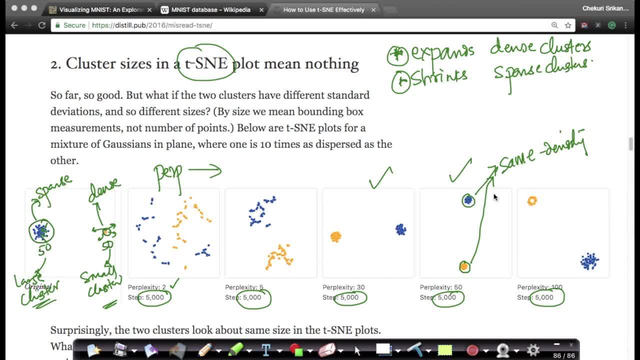 Imagine if you're shown only this. One conclusion that I could have come to is: oh, that okay. my blue points are here, my orange points here. they're well separated, number one, number two- Oh they're also. they also roughly have the same density. 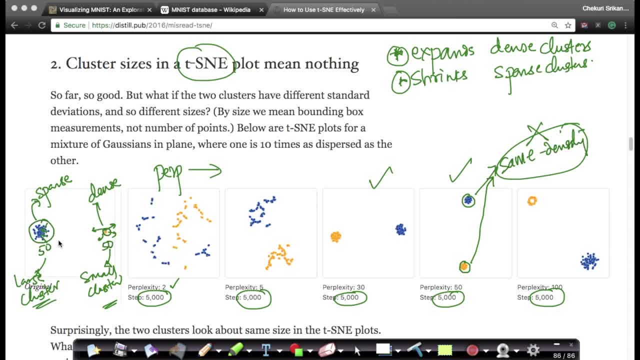 No, I can't come to the same density conclusion because t-SNE tends to- tends to expand dense clusters and shrink sparse clusters, So I cannot say anything about cluster size. Okay, This is very, very important, Okay. having said that, 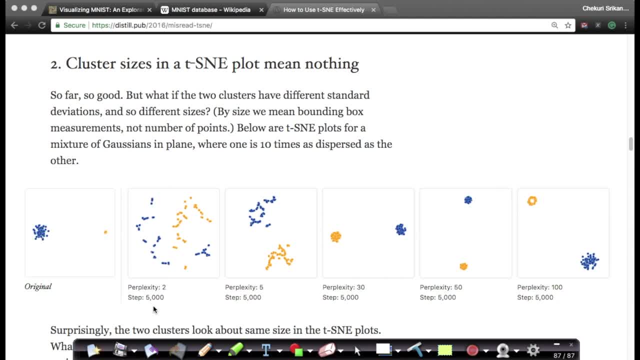 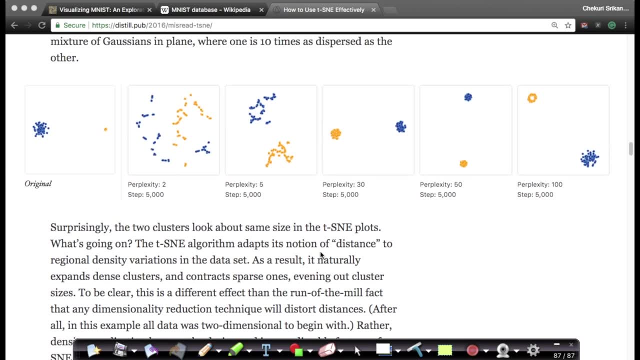 so this is one of the drawbacks of t-SNE, by the way. Now let's go and see some other examples. This block is terrific, as I've told you. Oh, there is a. we cannot also see relative sizes, right? 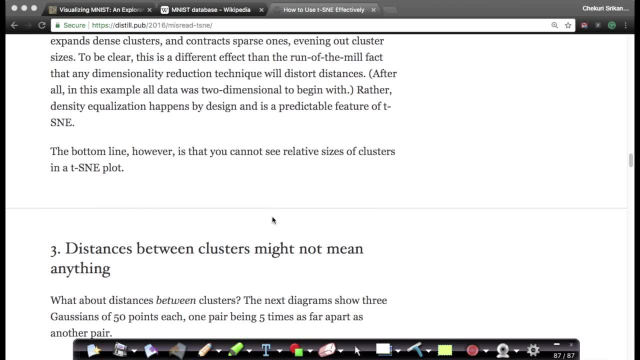 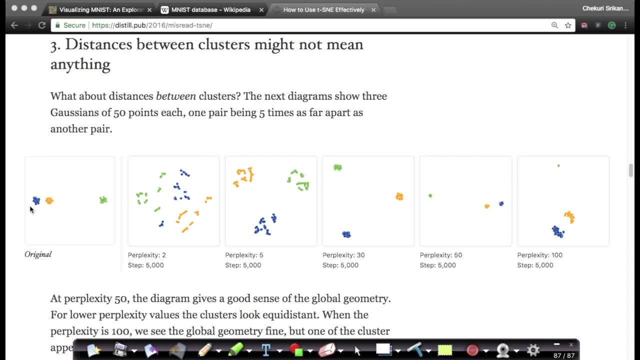 So exactly this point, right. So let's go further. This is a very, very interesting example. This example is mind-boggling. Suppose if I have three groups of points, okay. Now, in this case, what I'm doing here is: 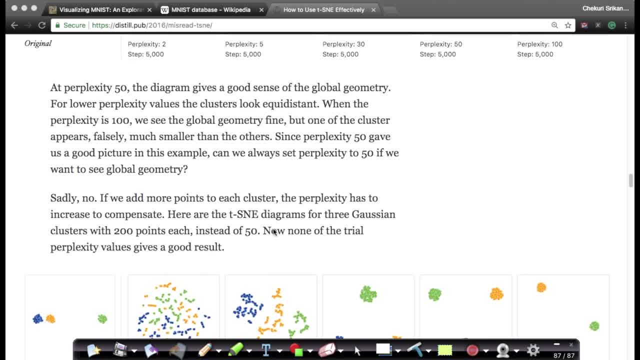 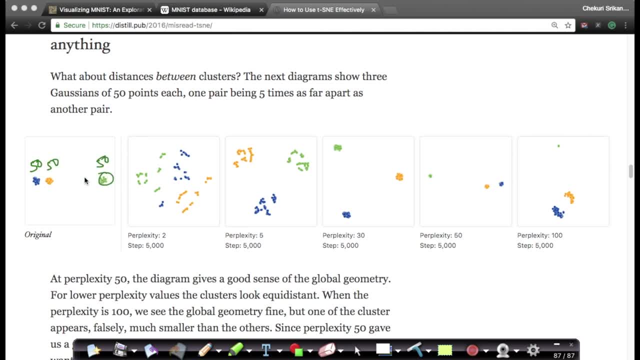 one second, sorry. Okay, imagine if I have three groups of points, 50 points each. I have 50 points here, 50 points here and 50 points here. Now you'll notice that between these two clusters, this distance- let's call it D1, is much lower than D2.. 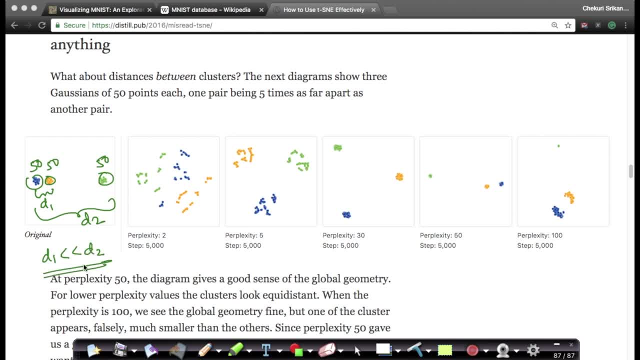 D1 is much lower than D2,, much smaller than D2.. So if I have a structure like this, where I have two groups of points, so two clusters which are close and the third cluster far away right, One of the problems that happens is: 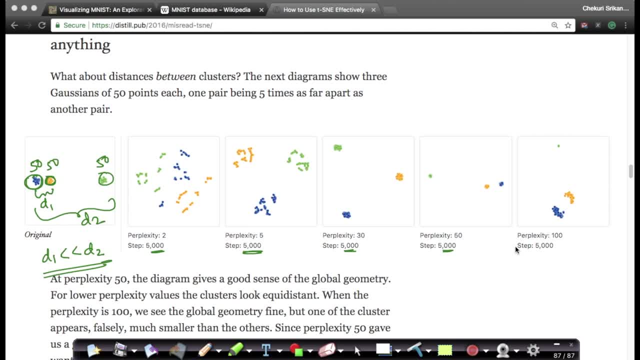 see, I'm keeping my step size fairly high, right, Even for higher values of perplexity. even for higher values of perplexity, only at perplexity 50,. this distance is much lower than this distance, But in this case the distances are almost similar. 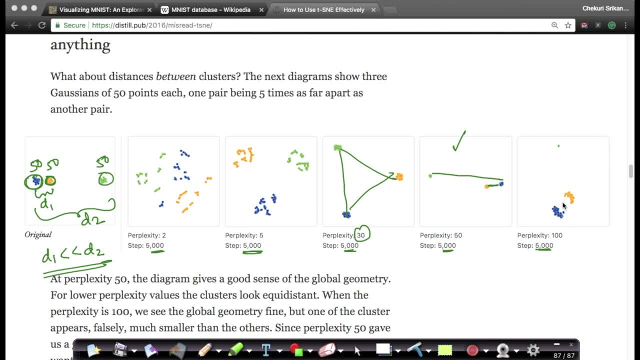 Of course, when I go to 100, the whole thing goes crazy. okay, because this has become much wider or much larger cluster. This has become much smaller cluster. But one problem is: imagine if I was looking at perplexity 30.. 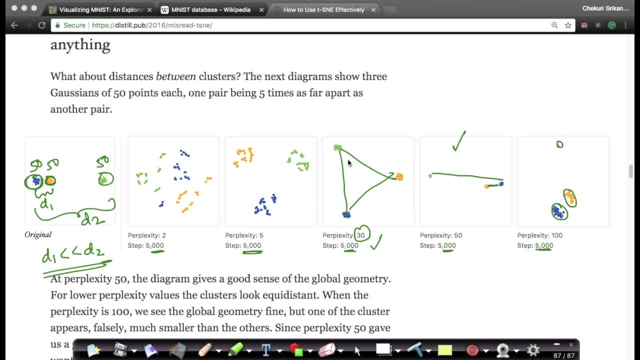 I could conclude that all these three clusters are at equal distance from each other, While in the real world, in the high dimensional space, in the original data they're not actually there. Your orange and blue points are much closer than your green points. 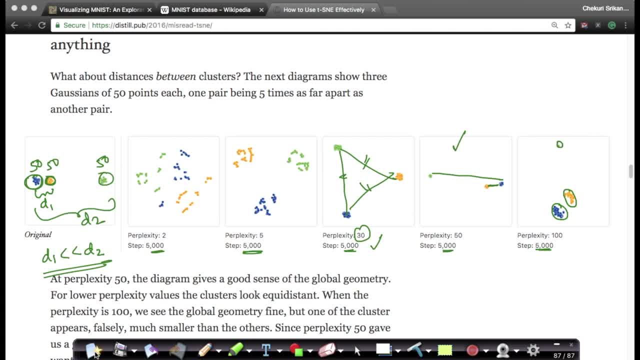 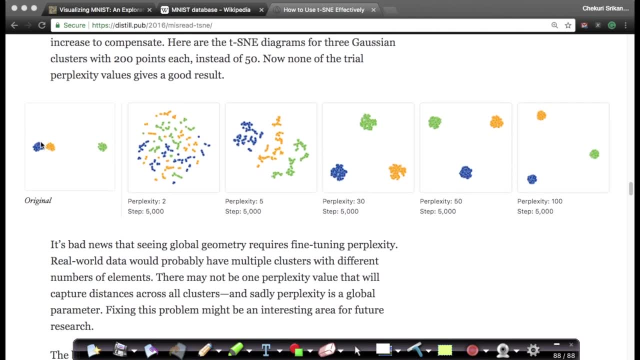 So this is the example with 50 data points. Now let's increase the data set and see what happens. This is a better example In this case. what they've done here is they have taken 200 points each, So you have 200 points of blue, 200 points of orange. 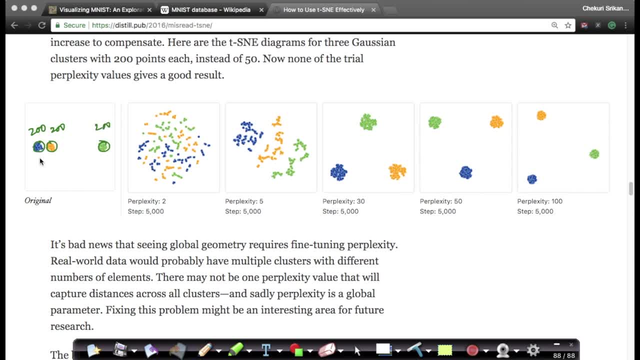 and 200 points of green instead of 50 points And of course this distance d1 is much less than this distance d2.. Now comes a problem, So I've kept my step or number of iterations fairly large. Whether I take perplexity equals. 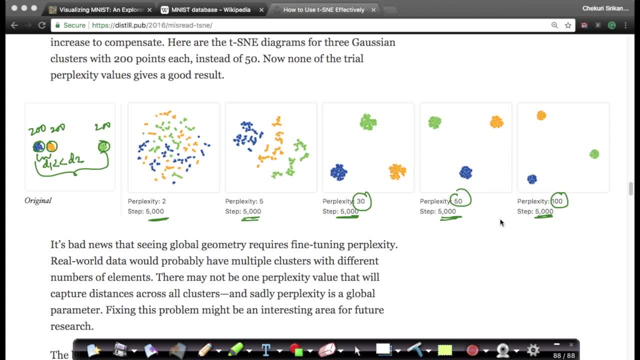 to 30,, 50, or even 100,. this shape that d1 is less than d2 is not being preserved. In this case, all three of them are roughly at the same distance, Similar thing. So what t-SNE is not doing is t-SNE does not preserve. 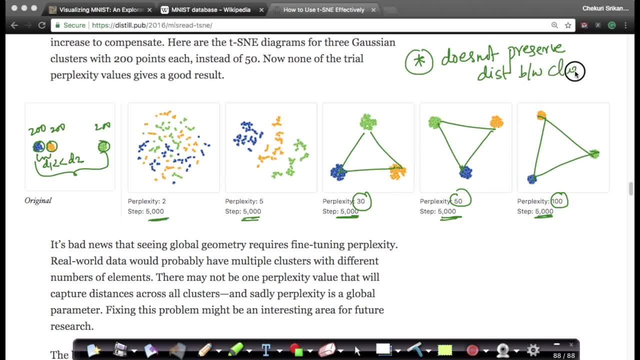 distances between clusters. We saw this example. This is 50.. In the case of 50, we at least got some good results when we had perplexity equals to 50, when we had 50, 50 points each. But when you have 200, 200 points here, 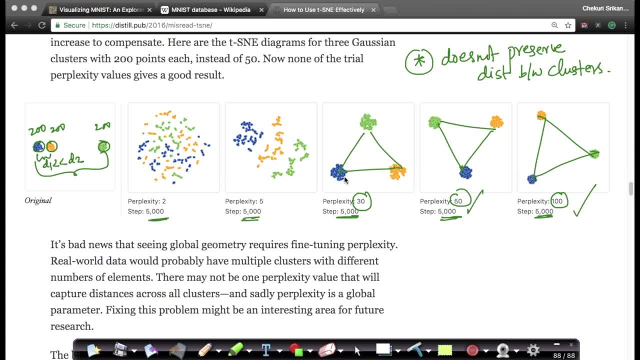 whether you put perplexity equals to 50 or 100, see the shapes are stabilizing. By just looking at these three, I could say yes, as I'm increasing my perplexity. this is all crazy. This is still crazy. 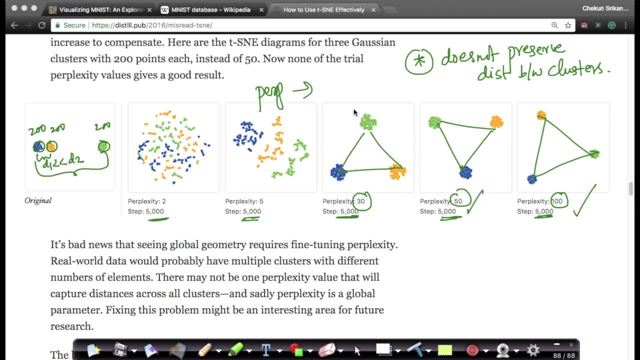 But as I go from 30 to 100, yes, the shape is stabilizing, So I could conclude that, OK, I have three clusters here in my original data And all of these three clusters are roughly at the equal distance. No, you can't conclude that. 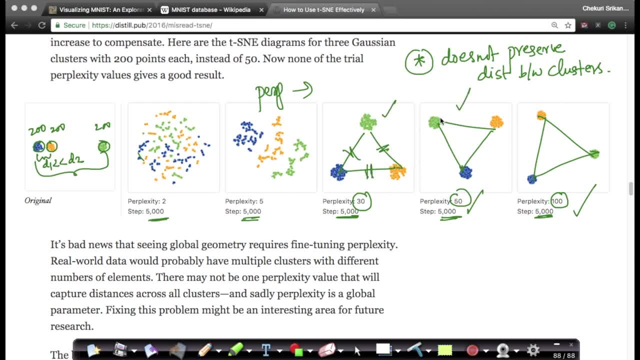 Because if you have this as original data set, this is what you could get as the result of t-SNE. So remember: t-SNE does not preserve distances between clusters. This is a very, very important observation or understanding. This is how not to misread t-SNE. 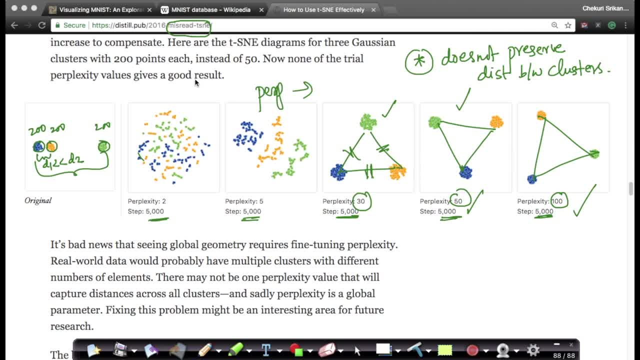 See the name of the blog itself says Misread t-SNE, So never misread t-SNE. These are all very, very interesting examples, geometrically showing what happens in various cases of t-SNE. OK, So now let's go down and see more examples. 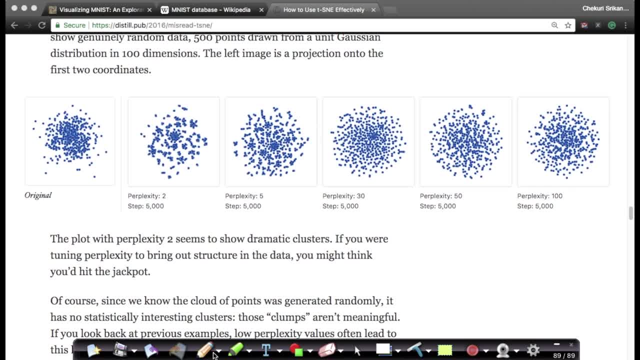 Oh, this is actually very exciting. So imagine if my actual data, my original data, is just random noise, just random bunch of points. OK, Random bunch of points. Now I'm keeping my iterations equals to 5,000.. And let's assume this data is actually. 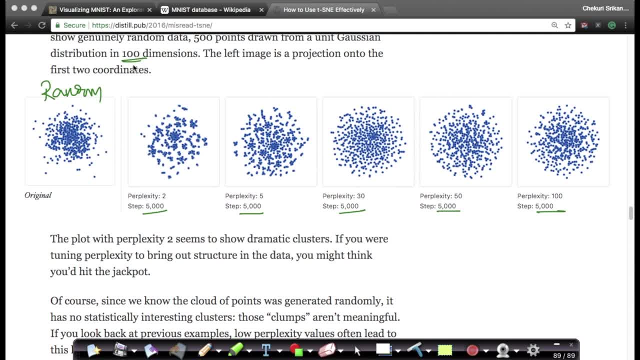 in some high dimensional space. OK, I think in this case they've taken 100 dimensional space, random points. Of course, I can't visualize 100 dimension, So they've taken some two dimensions and showing it to us that this is actually random. 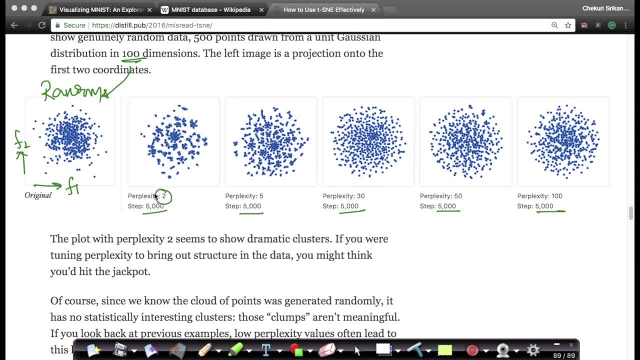 Now here comes. So when I have a small perplexity value, there is one problem when I have random data. See, one of the biggest problems in data science and machine learning is if you're making sense of random data, if you're making sense of junk. 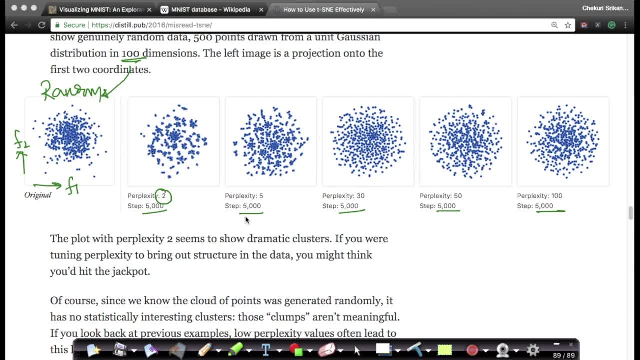 if you come to conclusions from junk, you're literally. it's an extremely dangerous position to be in. Never make conclusions from junk. So random data is junk. There is no structure to it, right, But when I keep my perplexity low. 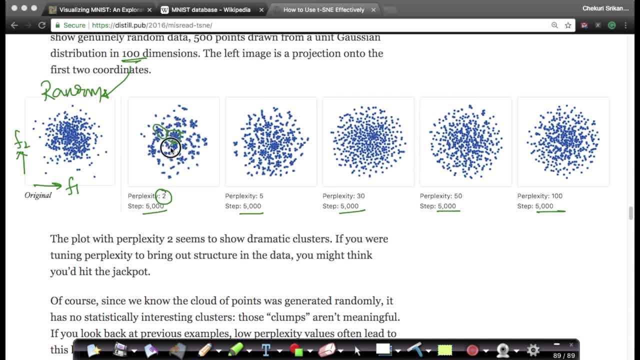 I start getting these small nice clusters when my perplexity is low, So I could conclude that, oh, there is this group of points here, There is this group of points here And there are small groups of points here. No, please never do that. 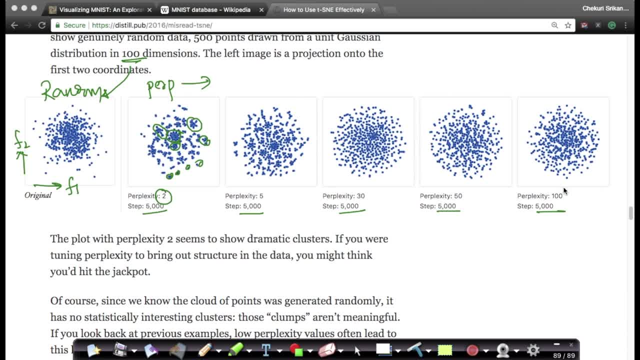 Always try your data for multiple values of perplexity. So the moment you increase your perplexity, this nice grouping is gone. And what happens now? And these are 500 points Originally, we have about 500 points here, 500. 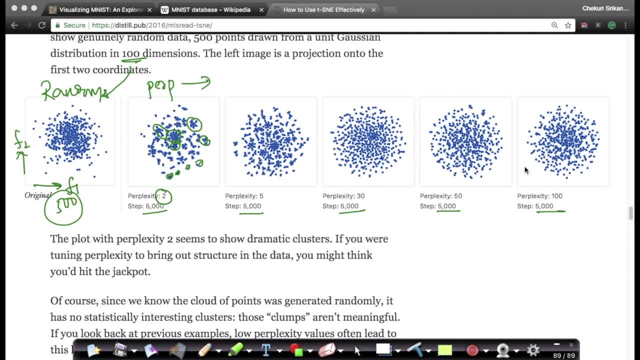 500 random points. So as your perplexity increases now, the data becomes more and more like random. So by the time you reach perplexity of 30 or 50, things have become. there is no structure here. It looks literally like a random bunch of points. 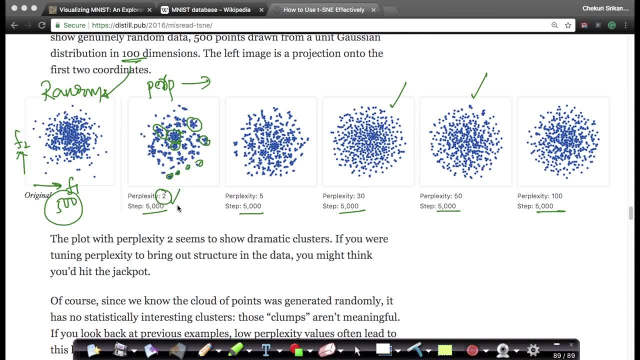 So never conclude that there is structure in data by just looking at one perplexity, especially small perplexities. Always look at more perplexity values, Otherwise you might end up in a case where you actually have random data and you're trying to make sense out of it. 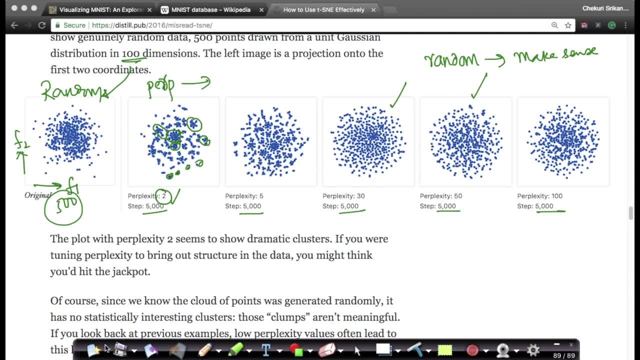 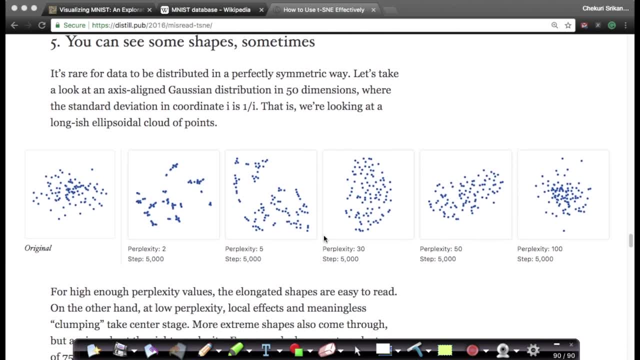 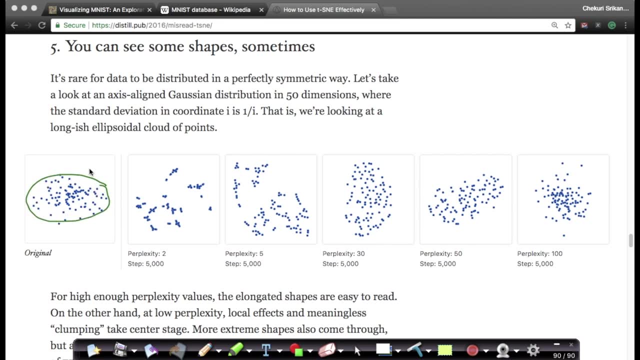 You might even come to wrong conclusions, which is extremely dangerous. Having said that, let's move on. Let's move on to. so. this is another very interesting example where I have data like this, I have like an elliptical data, And when I have small perplexity. 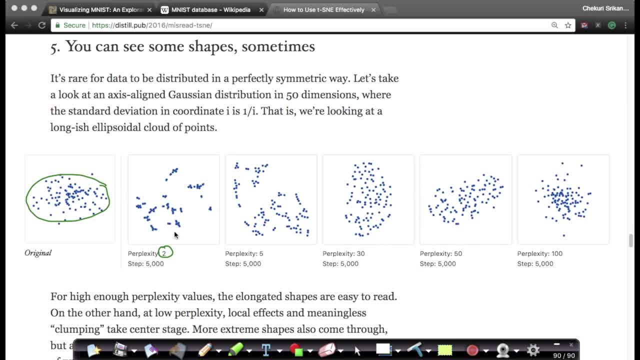 you can start seeing shapes where there are none. When I have small perplexity, I'm getting these groups of points. So again, the lesson, The lesson to be careful here is never just learn with a small perplexity, Keep increasing it. 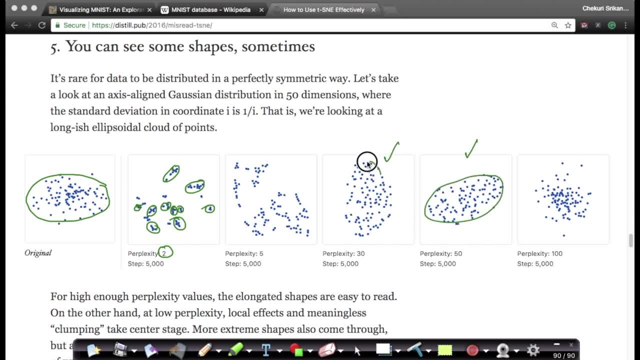 By the time you reach a perplexity of 30 or 50, the shape is becoming more and more clearer. But of course there are more points here in the center. Here all the points are almost equally spread Because we know that t-SNE the original data. 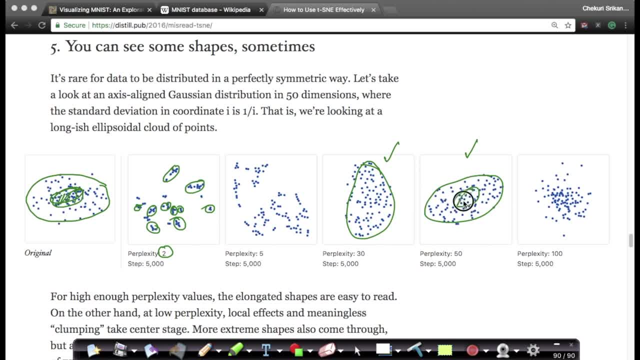 there are more points in the center here, But here the density of points is almost spread Because we know t-SNE tries to do this. We know internally that t-SNE tries to spread And it does spread out points evenly. So that's another thing. 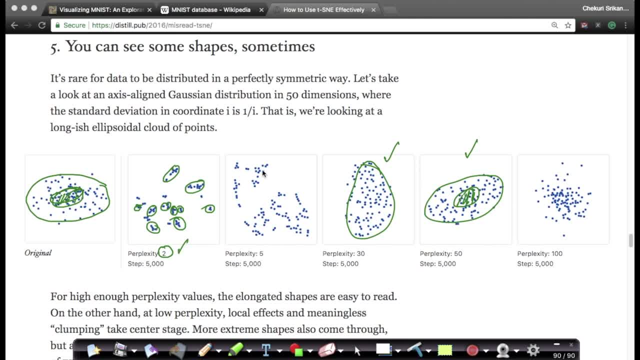 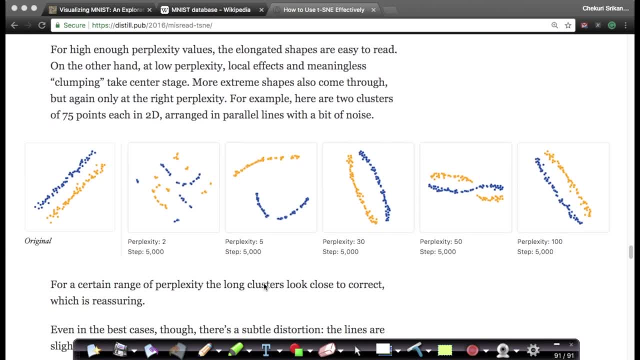 So never just look at small perplexity values or two or five. even in this case You could conclude that, OK, there are these nice clusters here, So never get confused by that. The next thing very important is: imagine. Imagine if I have a data set like this: 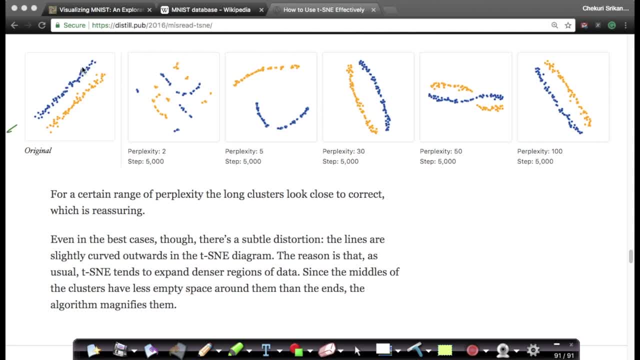 This is very, very interesting again. So this is my original data set: two lines of parallel two. So I have my blue points like a line And I have my orange points like parallel lines. These are called parallel line data set, the basic data. 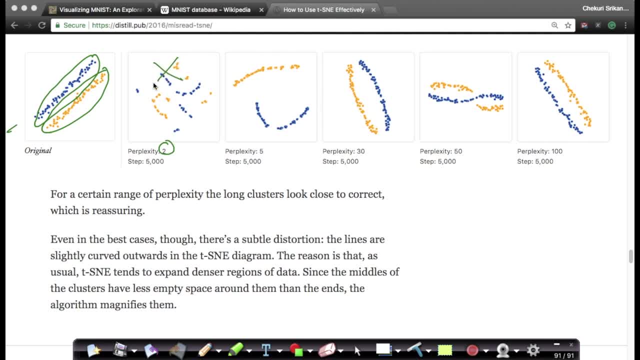 points which are parallel to each other. Now, when I have my small perplexity anyway, everything goes crazy. But even as I increase my perplexity here, I'm keeping my iterations equals to 5,000.. I could end up in a situation like this: 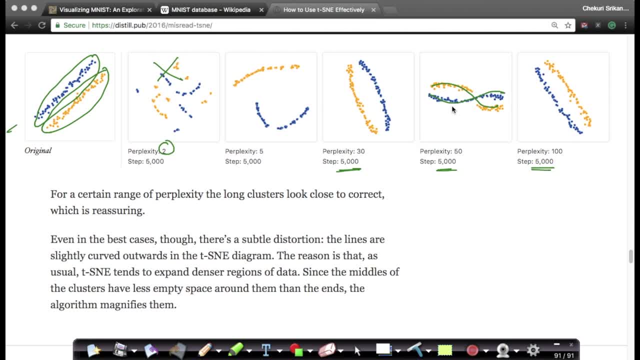 I could end up in a situation like this: So this looks like your gene-shaped data, But it's actually not your gene. So Always Change your t-SNE multiple times or increase the perplexity. So here, what happens is, as I'm increasing my perplexity, 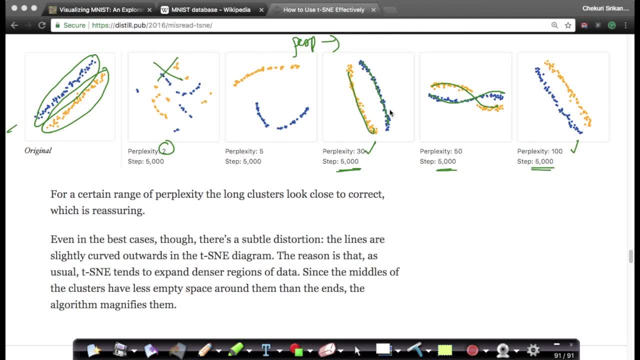 I got this almost good shape. I almost got a good shape And then it went crazy as I increased my perplexity- And when I made my perplexity equals to 100, it almost converged to the right shape that I'm looking for. 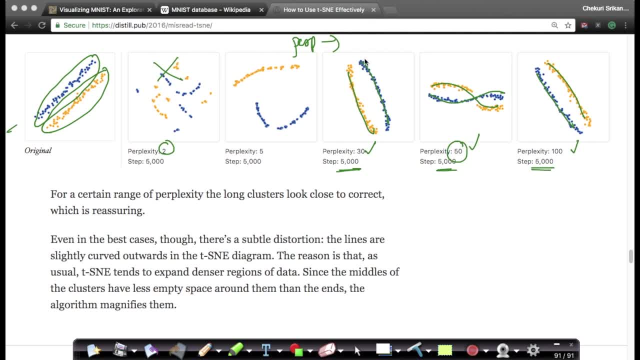 So whenever you get results like this, it's always good to rerun. See, that's why never draw just one t-SNE plot and come to a conclusion, Change perplexity, change step size and, third most important, always rerun. 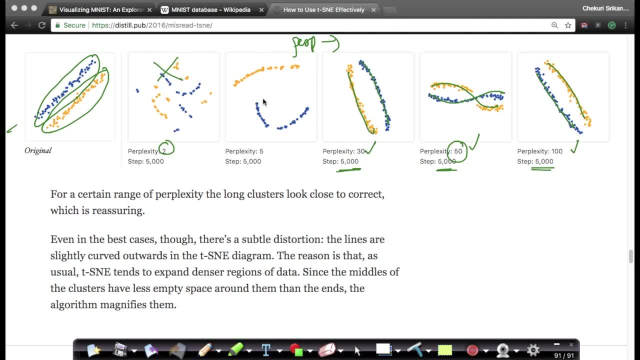 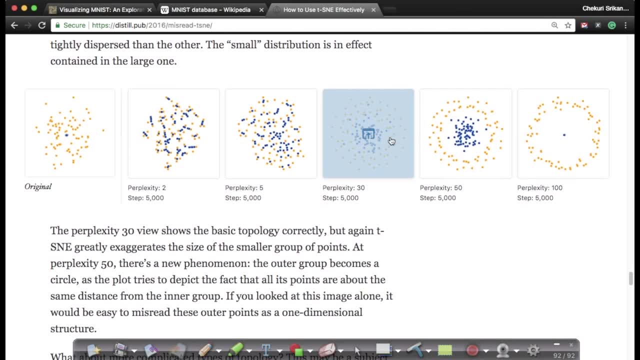 with the best perplexity and step that you've got, or the number of iterations that you've got. Having said that, let's move on now. This is much more exciting. These are called topological shapes, So imagine that I have a bunch of blue points. 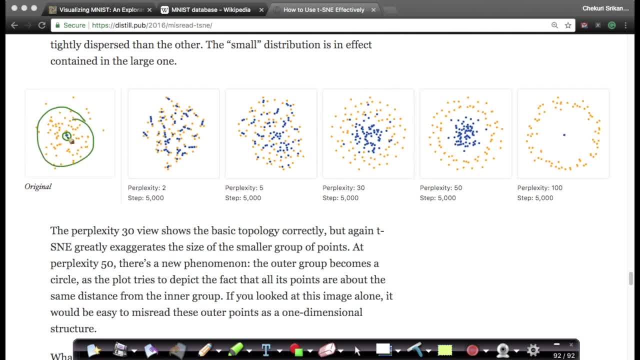 inside my orange points. Suppose if I have a bunch of blue points which are very, very dense inside my orange points, when perplexity is small anyway, it makes no sense. But as I keep increasing my perplexity I will start seeing the shape eventually. 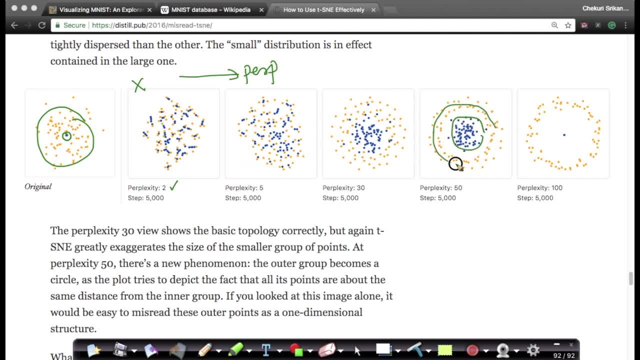 where all my blue points are inside my orange points. But as soon as I increase my perplexity further, I'm losing. So I'll not get exactly this shape, but I'll get a sense that, OK, blue points are inside my orange points. 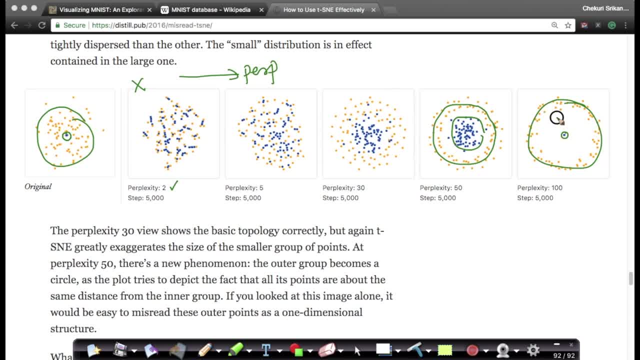 But I'll not get the perfect sense. See, this shape is not exactly the same as this shape or this shape, So it can- perplexity of 30 here, or perplexity of 50, can- show the basic topology or geometry here. 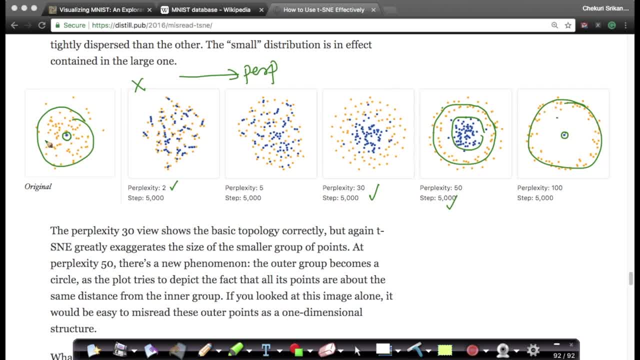 Topology is the study of shapes. in mathematics It's a very, very wide area. So here the shape is called containment, because these points, these blue points, are contained within my orange points. Here by the time I have my perplexity 30,. 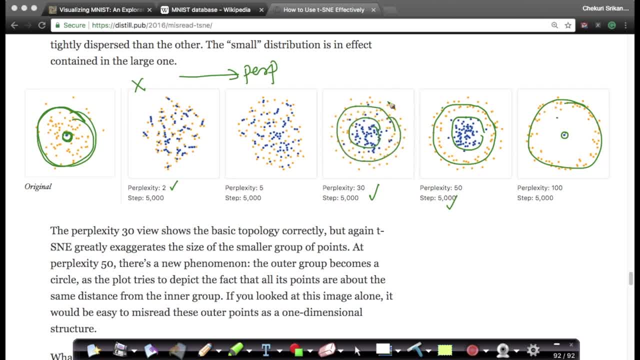 I'm getting a sense of what's happening, that all my blue points are inside my orange points. But as I increase my perplexity, I get a sense of what's happening without exactly replicating this result. PC never exactly replicates the result. 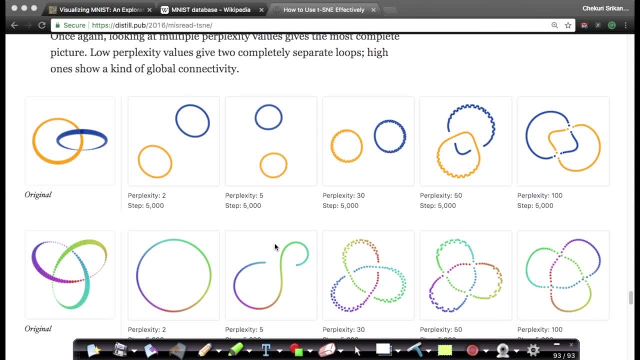 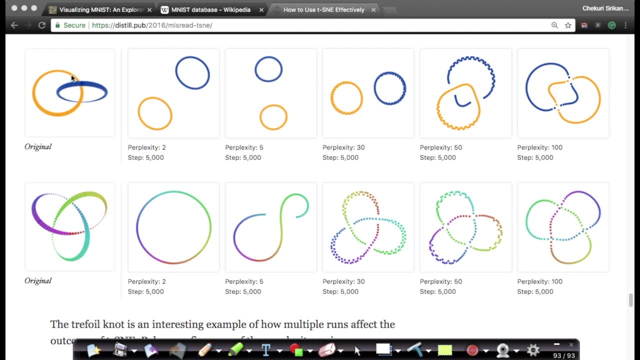 OK, So that's an important lesson there. Now these are called interlocked rings, So these are more complex topological structures. This is a shape where I have two rings interlocking each other. Now what happens here is when I have small perplexity. 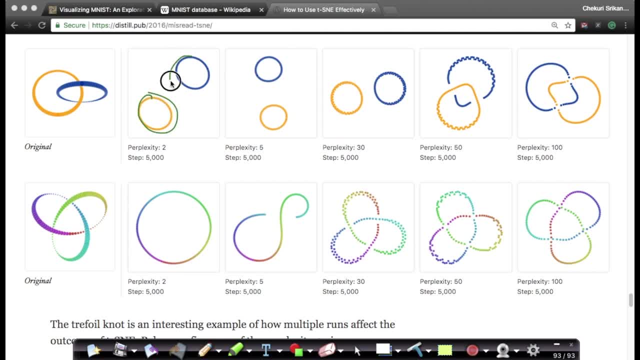 I just get disconnected. I just get disconnected circles, But as I increase my perplexity, eventually I'll reach a stage where my points show this interlocking structure of the data. Similarly, if I have this, this is a very, very complex. 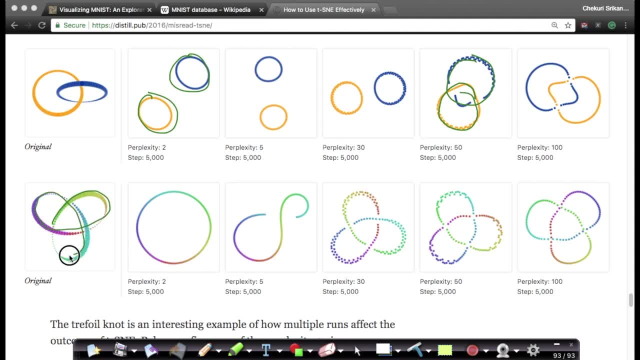 knot-like structure. So this knot-like structure is like this Very interesting knot-like structure in topology: When my perplexity is small, I get nothing. But eventually, as I increase my perplexity, I start getting this shape where all of my violet points. 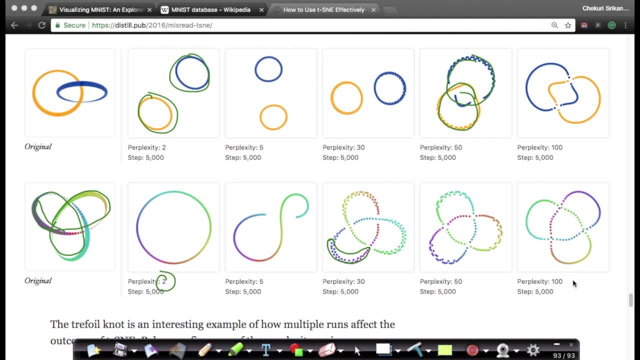 here get grouped together. I get a sense of the geometry as I keep increasing, or I get a sense of the shape or topology as I move towards this. So don't worry if you don't understand what topology means. Just remember that topology is a study of shapes. 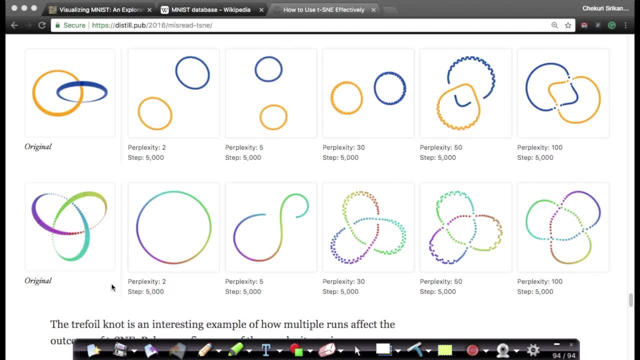 Am I preserving the shape? Yes, more or less. OK. So this is again. by the way, this structure is called the trefoil knot- Trefoil knot, sorry, This is called the trefoil knot. It's a very, very interesting shape. 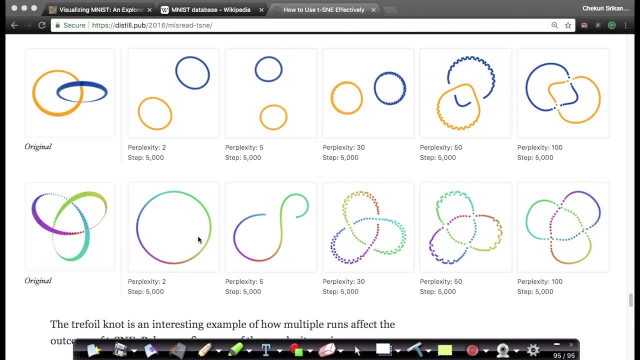 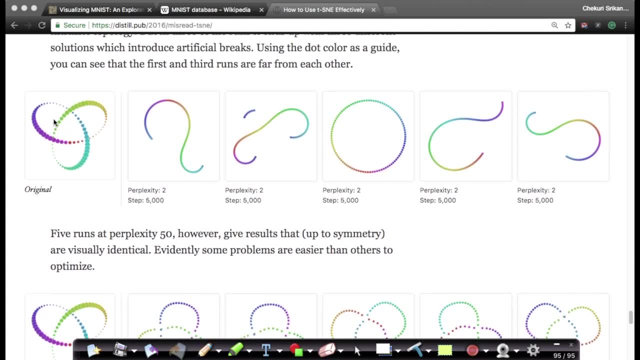 in the study of shapes, which is the area of topology. OK, having said that, now comes the interesting part. So if my actual data was my trefoil knot, if I have 5,000 iterations every time and remember I'm running, 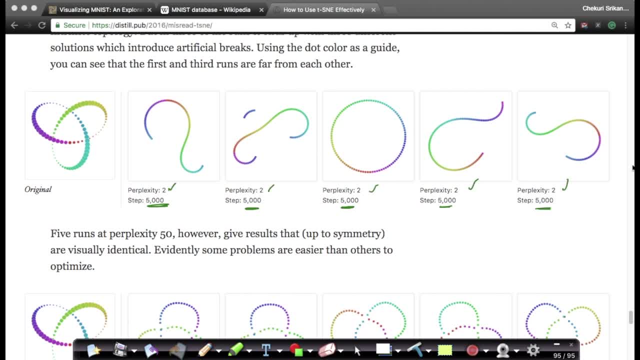 perplexity equals to 2.. These are basically multiple runs of t-sling. This is my original data, So with every run I'm getting a different shape. What is a lesson from this? It means perplexity of 2 is the wrong thing. 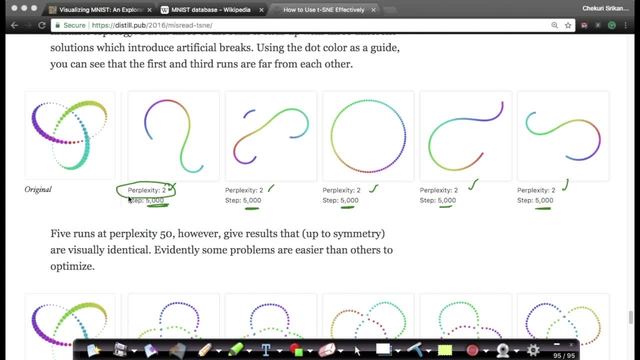 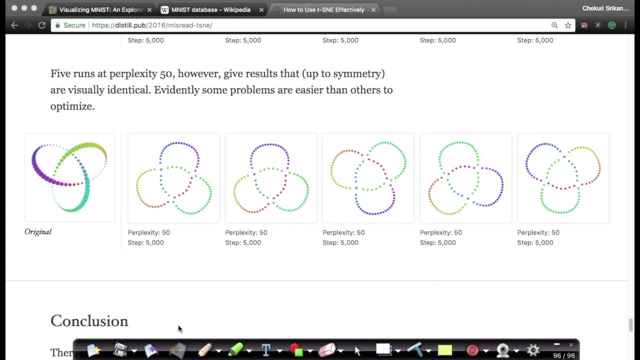 because every time I run it I'm getting a completely different result, which means this perplexity 2 is no way the right, stable answer right Now. instead, if I run this, if I run the same thing with, let's say, this is my original data. 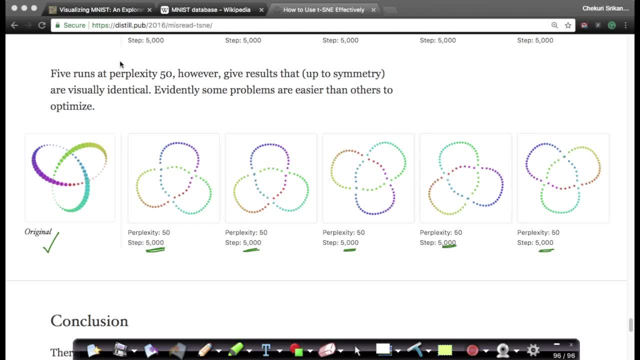 I again run for 5,000 iterations of 5,000 steps Instead of 2, like above. if I keep perplexity 2, like above, instead of 2, like above. if I keep perplexity 2, like above. 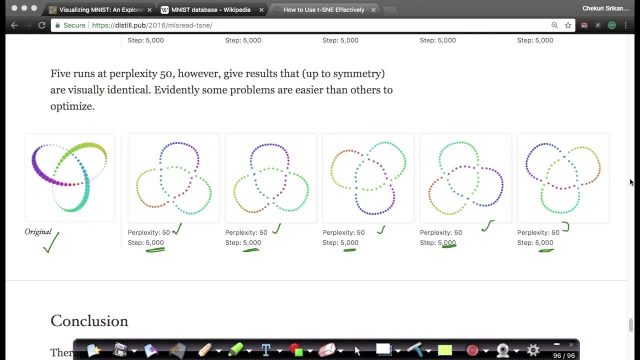 instead of 2, like above, if I keep perplexity 2, like above, if I keep perplexity of 50, and if I run it five times, this is the outcome of five times running it five different times there. 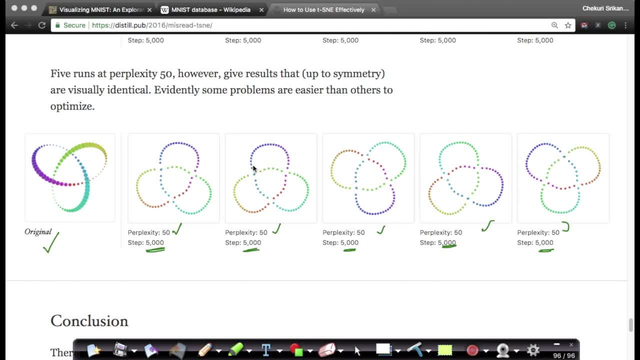 is a slight difference, For example, between this and this. your violet points are here. In this case, your violet points have gone down, But the shape is more or less well-preserved, right. In this case, your violet points have come to the right. 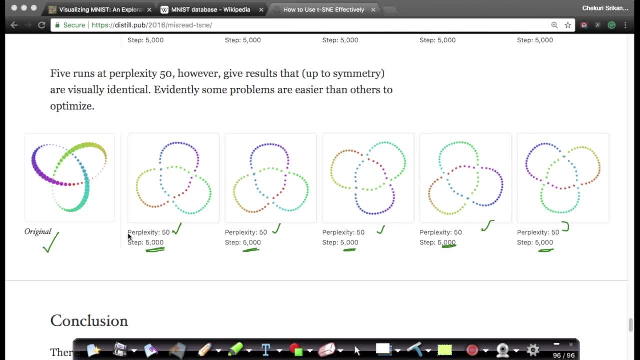 In this case, your violet points have come to the left right. So by running the same t-sling algorithm multiple times with same value of perplexity and step or number of iterations- if this is the shape is stable- shape could rotate. 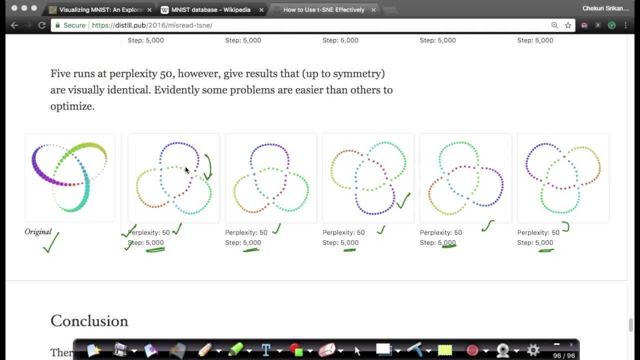 So this probably rotated like this and created this. Shapes can rotate, That's perfectly OK. Or if I rotate this slightly on this side, I get this shape. Or if I rotate this like this, I get this shape. That's perfectly OK. 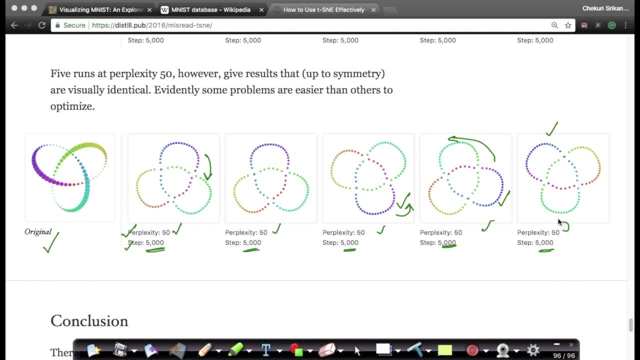 So by running my t-sling algorithm multiple times, if I can understand, if my shape is roughly the same, then I know that this perplexity value and this number of iterations is stable. So the most important lessons to learn for all of us. 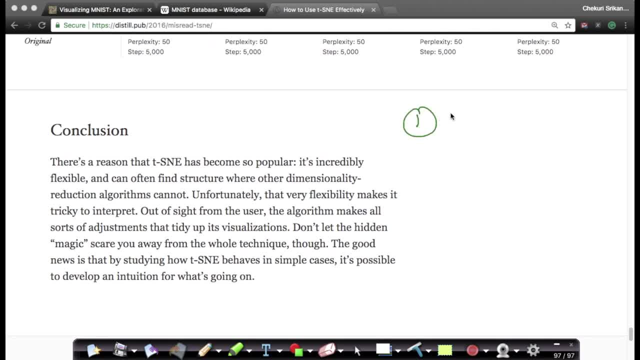 the most important lessons are: always run your steps or number of iterations till the shapes stabilize. This is the first thing. Second is try various values of perplexity. If you have n points, always try to keep it less than n, But try to do it between 2 to n. 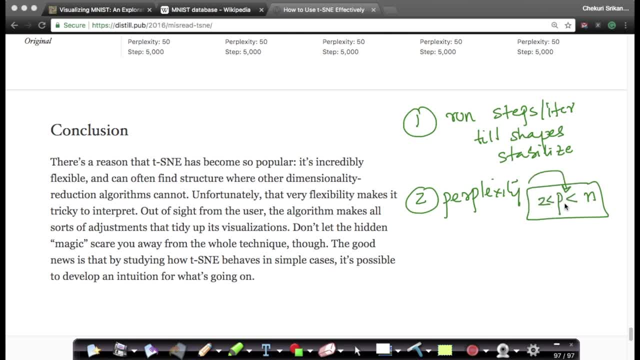 OK, Try to keep your perplexity. OK, try to keep your perplexity between 2 to n And see how the shapes are changing. never run t-SNE once. The most important lesson: never run t-SNE just once and start reading it. 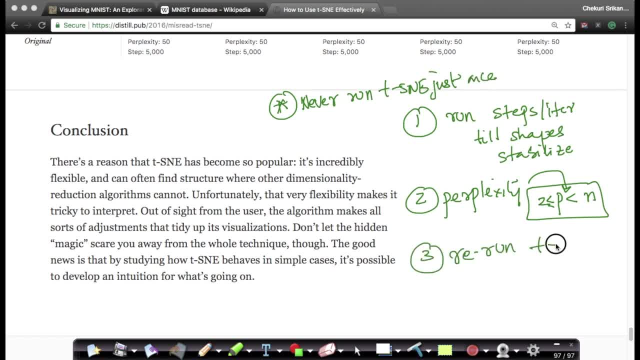 Third, rerun your algorithm. rerun your t-SNE with a perplexity value and a step or the number of iterations multiple times. just rerun it multiple times and notice whether the shape is stable or not, As we saw with the with the trafoil knot. These are the most important lessons. 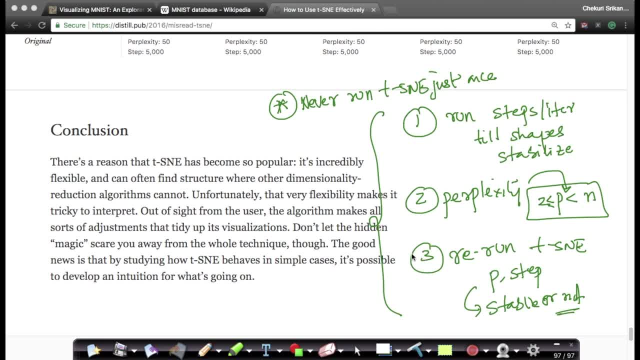 of t-SNE. Never run your t-SNE just once. It's a terrible, terrible idea And, thanks to folks behind distilpub, it's a terrific blog which gave us all of this nice intuition And, as I promised you, let's just go up. You can play with this data for a very long. 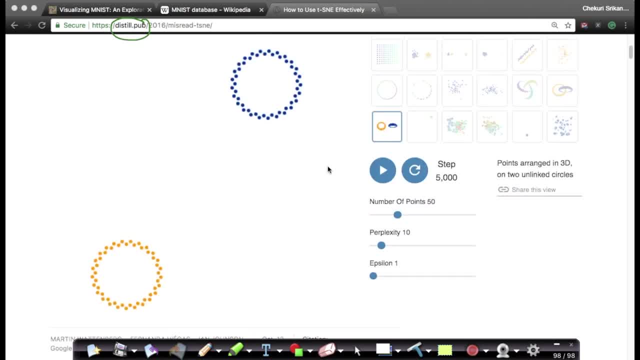 time. So you have all this. So if I just go to the top of this page, I have all of these shapes. I have my trafoil knot here And I can say I want a perplexity of, let's say, 50,, 60,. let's say It's going crazy. now 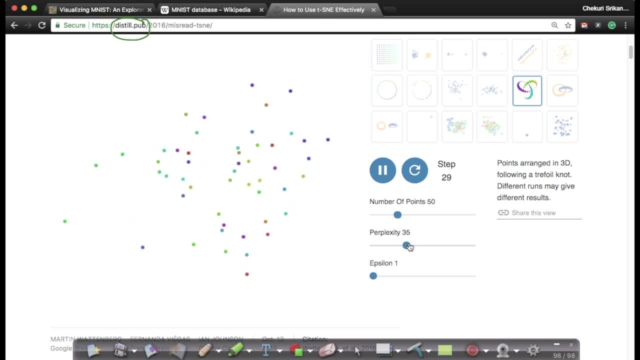 Because my perplexity is just too high. What if my perplexity is slightly low? Yes, as my perplexity is slightly low, by the time I reach 1000 iterations, I got the rough shape Epsilon. forget about it, Epsilon. here is another parameter, Don't worry about it. 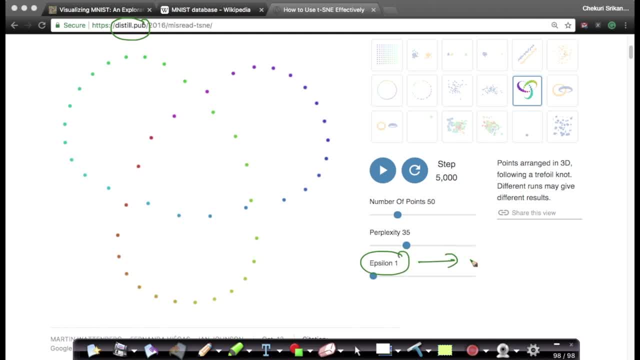 It basically tells you how fast you should change, how much should you change from one iteration to other iteration. This is mostly an optimization parameter which you can ignore. Just keep it at some reasonable value. I kept it at one, but you can just fix it at any value and just read on it. The more this 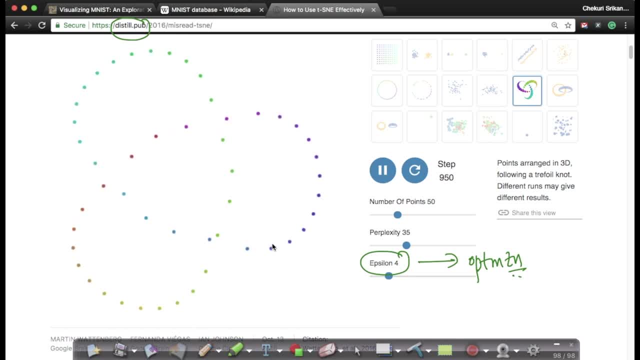 value is, the faster your data will converge. That's all, which means the more epsilon. as epsilon increases by the time you reach a smaller number of iterations, you'll solve the problem. That's it Not always guaranteed. There's some catch.